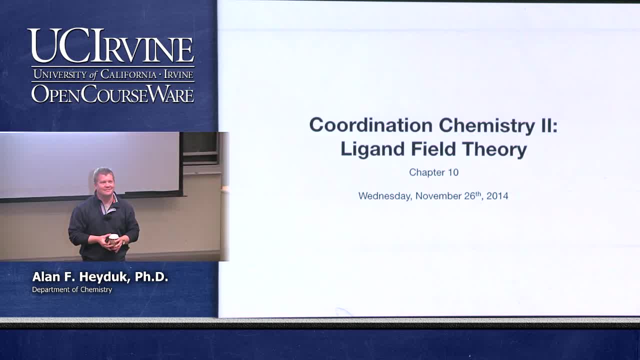 half of you Who's going the furthest You are, It might take. I mean, if you walk really slow, though, it may take you a while. Is anybody leaving the state of California? Wow, Somebody needs to get out a little bit more often. There are other places. Nobody Into. All right, okay. So just across the border, though That's a different country, though You need a passport for that. Some may say I'm from Ohio. some may say you should need a passport to go to Ohio because it's like a different country, But I'm not traveling. 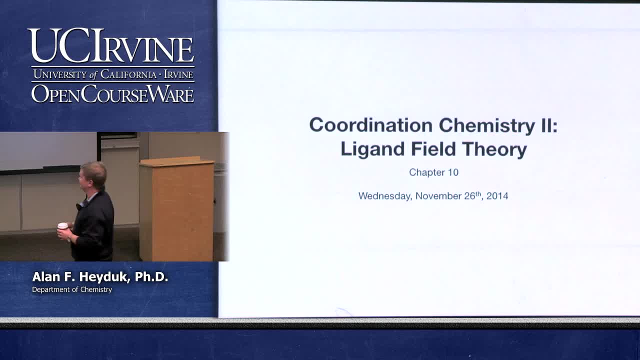 so I'm cooking Thanksgiving for my in-laws. Aren't I a great, Great husband? Okay, So chapter 10.. Oops, I should turn this on. There we go, All right. So we mentioned that. did you have a question? 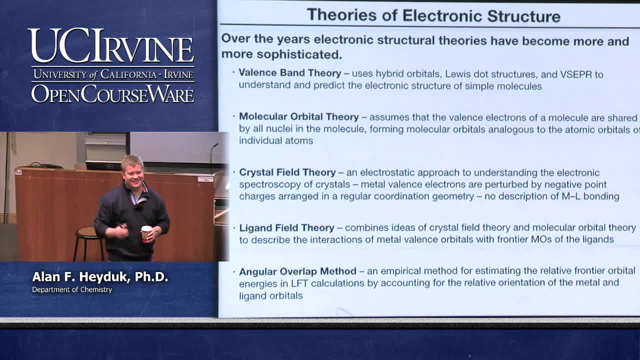 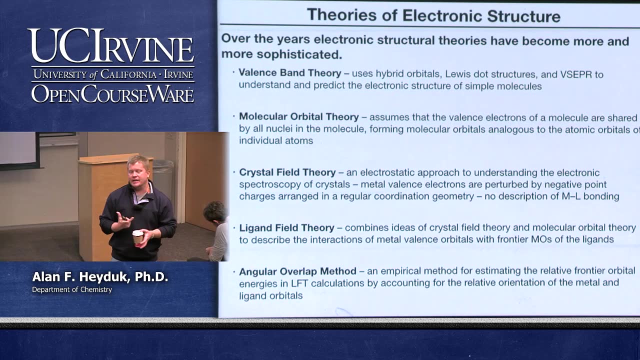 No, no, I'm good, Are you sure? Yeah, You raised your hand though. Okay, You're good. Okay, We're all. okay, Yeah, Okay. So chapter 10, electronic structure of coordination complexes. It turns out that it's more difficult. 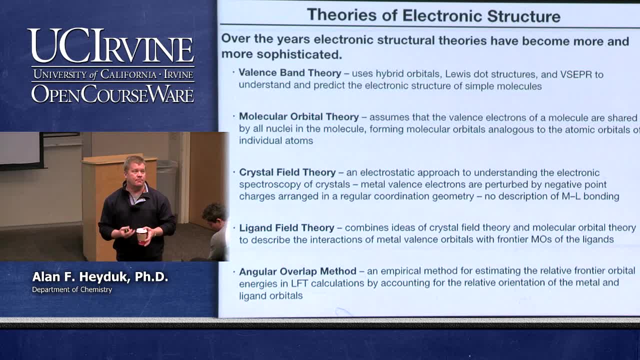 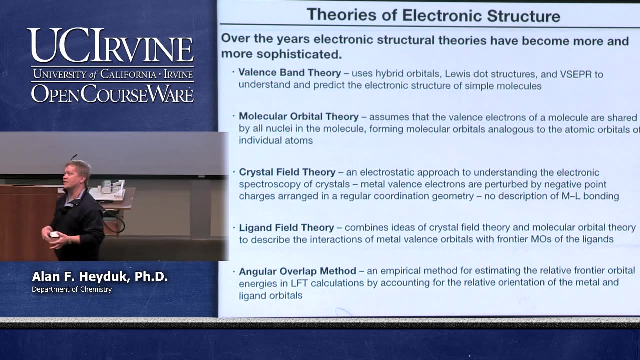 to understand the electronic structure of coordination complexes. The models that we use are more sophisticated, which we're going to learn over the course of the next couple of days- And even though the models are more sophisticated, they're also more prone to not getting it quite right because, again, the problem just gets much more difficult. It. 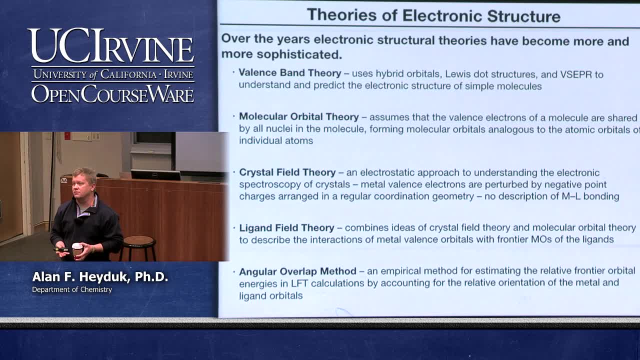 It turns out that when you're dealing with a molecule like H2,, eh, you know, fairly easy to get the electronic structure right. When you're dealing with a molecule like a heme porphyrin, and it's got, you know, 127 atoms and whatever. 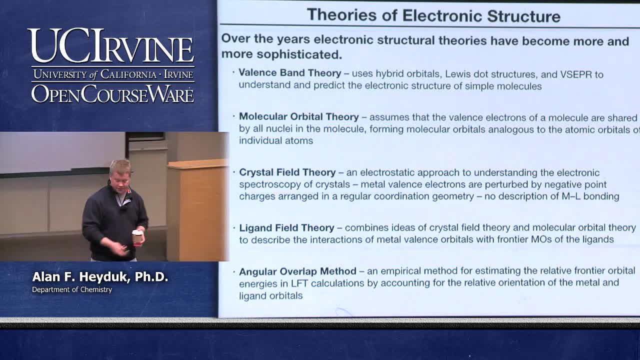 it gets a little bit more difficult. So we have these more sophisticated models to help us try and understand, do what I like to call a back of the envelope type calculation. So computational chemistry is really powerful, but not all of us carry around a computer in our back pocket. 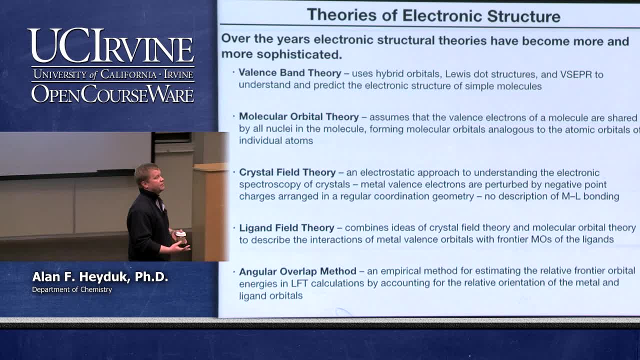 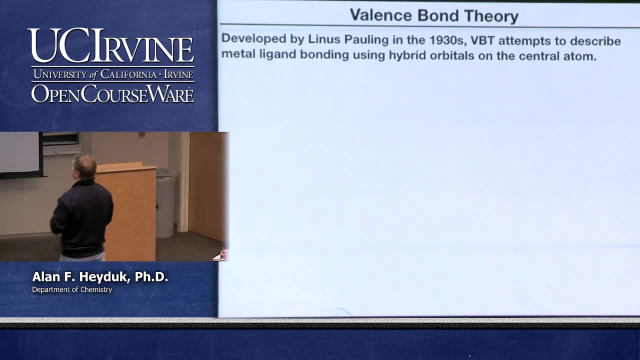 And even if we did, we wouldn't want to run a calculation. So it's very useful for you to be able to sketch out on a piece of paper and get an approximation to the electronic structure of a complex. So the models that we use they start in the same place. 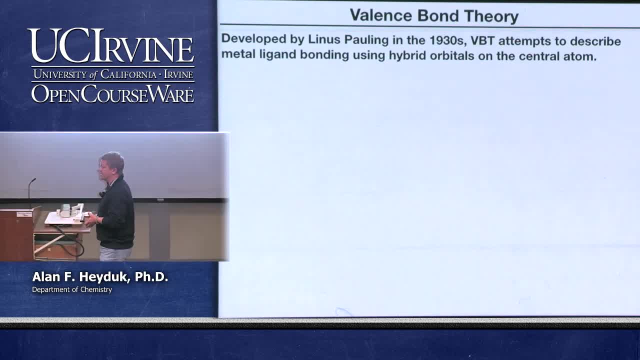 that we've learned for all since freshman chemistry. So Valen's, Valen's bond theory was developed by Leinart Linus Pauling. actually, Linus Pauling was the answer to a Jeopardy question this week. 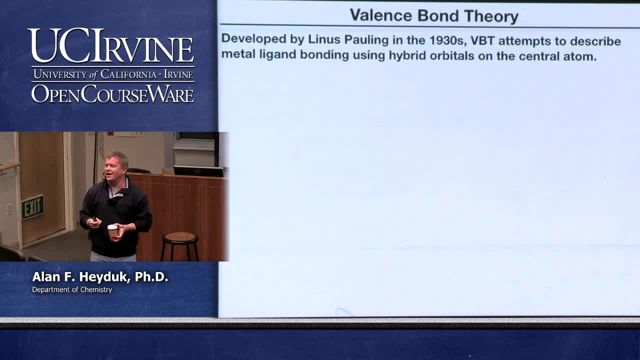 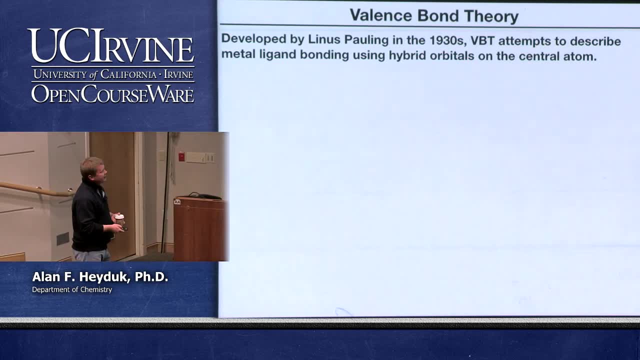 It was chemists with the letter P or something like that, And so he's. he's the one that's won that won two Nobel prizes, So that's not so bad. But Valen's bond theory attempts to describe the electronic structure of a molecule. 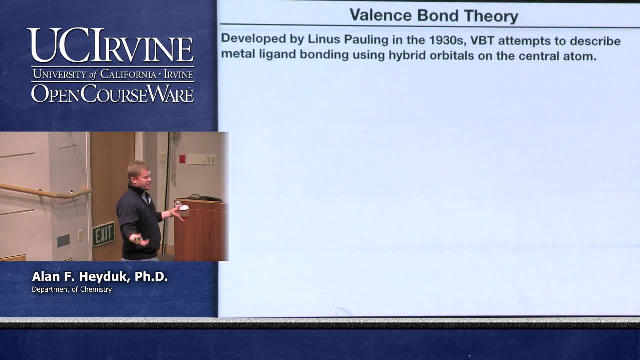 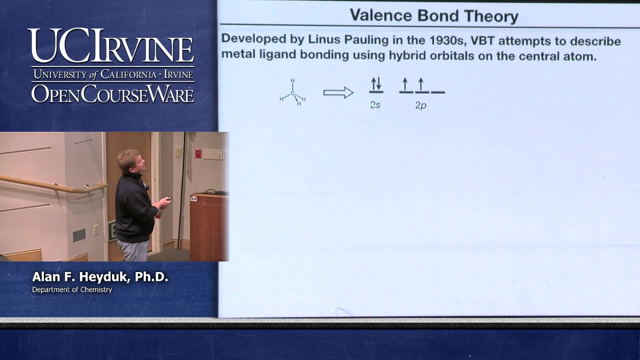 by using, by basically saying that the, the Valen's electrons stay associated with their, the original atom they came with, And then you use these hybrid, hybrid orbitals, okay, And so it works remarkably well. for organic chemistry, We know, for a molecule like methane, we take the carbon. 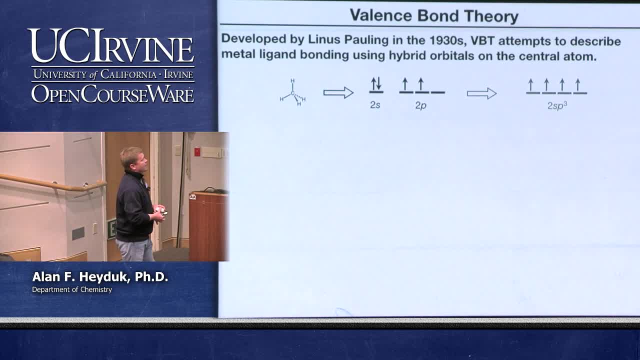 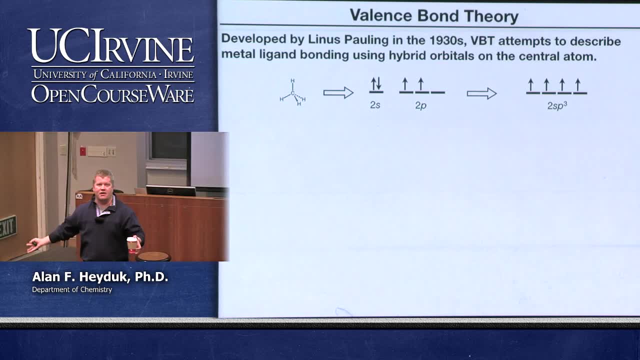 which has a 2s orbital and three 2p orbitals, And- and we we do this mental exercise of putting them into a meat grinder- and and and spitting out four equivalent orbitals. sp3 hybridization: It allows us to take the two electrons that are: 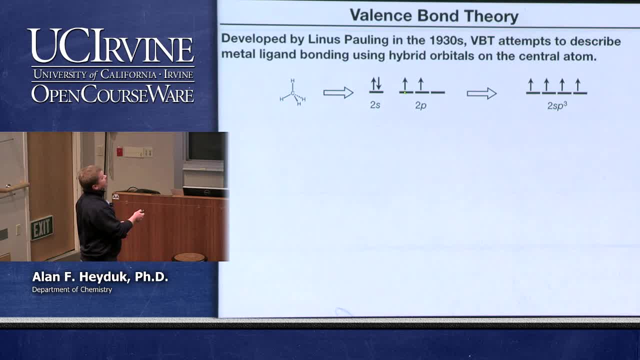 in the 2s orbital and the two electrons that are in the three 2p orbitals and put them all spin up into equivalent sp3 hybridized orbitals. Then, when we bring in our four hydrogen atoms, each which has one electron, 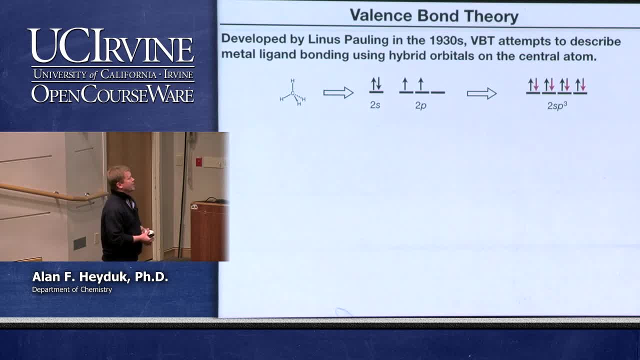 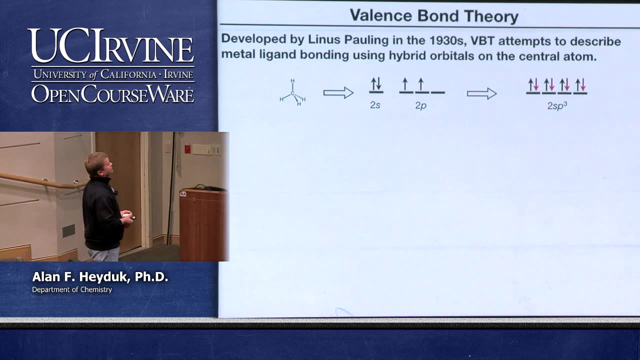 we can form four equivalent CH bonds. Now, for reasons that are beyond the scope of of today's class, this is completely wrong, But nevertheless it it works for certain things and it helps us predict that methane should have that. methane should have four equivalent CH bonds. 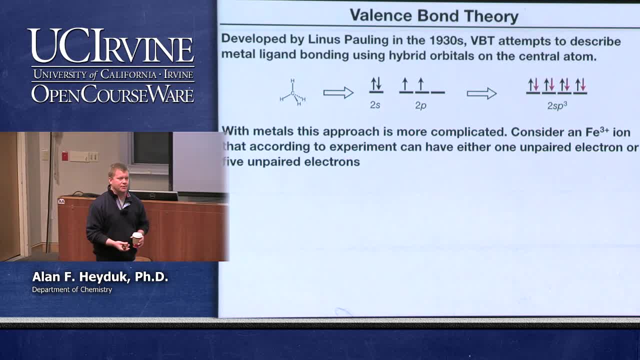 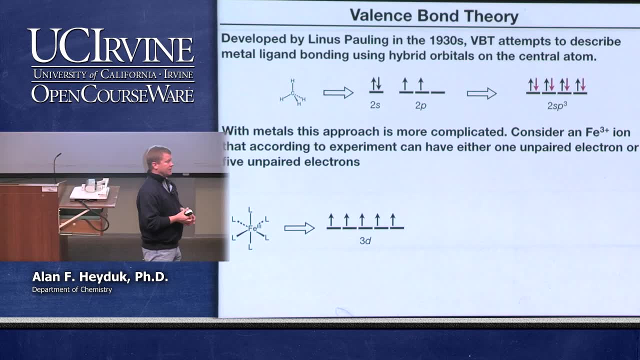 So when we, when it comes to transition metals, things get a little bit more complicated. okay, And we can see that if we just consider a simple octahedral iron 3 compound. okay, We know that if we have an iron 3 compound, 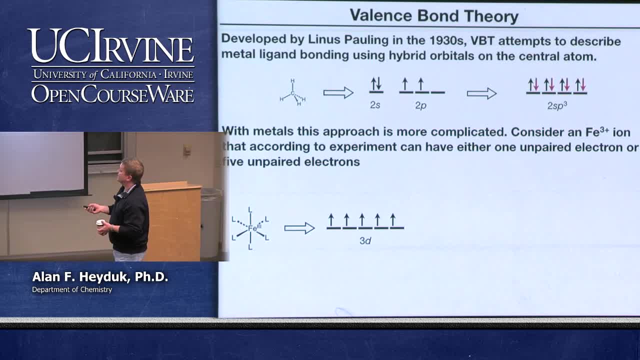 we learned how to count these electrons in freshman chemistry. It's a, a 3d5 electron configuration. We know from the Pauli exclusion process, the Pauli exclusion principle and Hund's rule that we put these five electrons into the 3d orbitals. 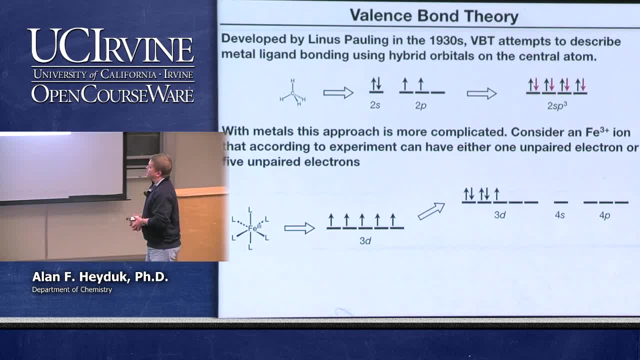 They all go in spin up. So then, if you want to use this kind of valence bond theory approach, you have to think about how you're going to make bonds to these six ligands okay, And we know that we can treat ligands as Lewis bases. 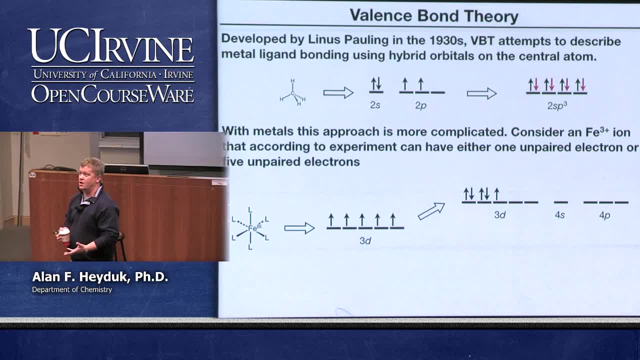 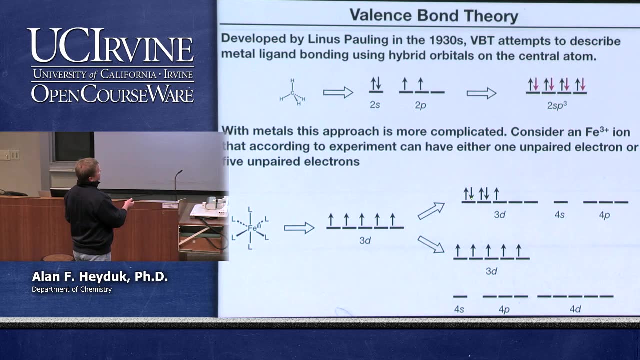 which means they're bringing a pair of electrons, which means we need enough metal-based orbitals to hold a total of ten electrons, And so one way you can do that is to put all five electrons into the 3d orbitals and start pairing them up. 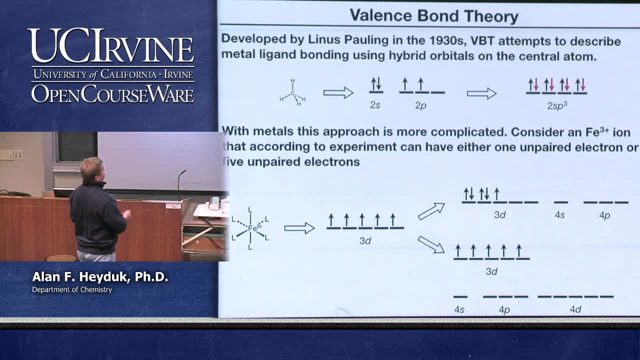 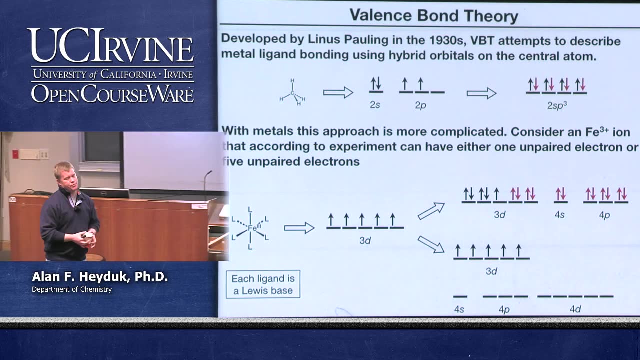 Or you can put them into the 3d orbitals like this, following Hund's rule and and Pauli exclusion principle, all spin up. These would be termed the the high spin configuration and the low spin configuration, And so then what we what happens is we can bring: 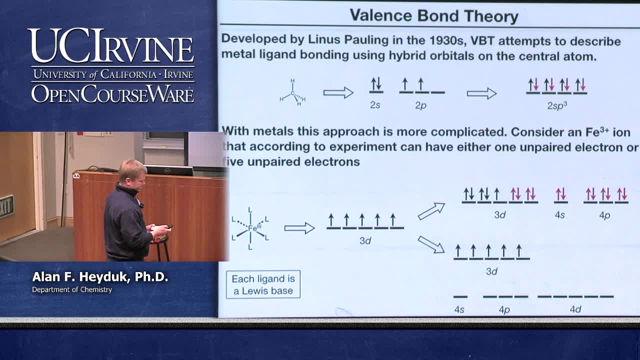 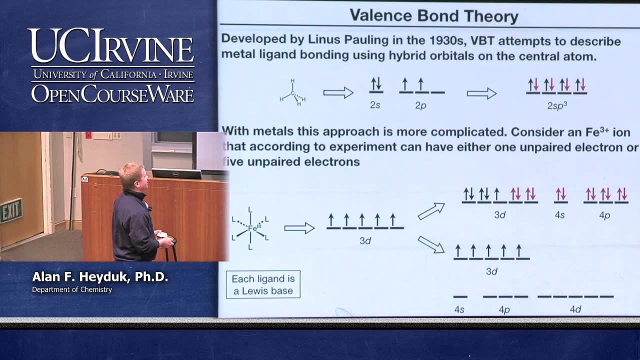 in our six pairs of electrons for the Lewis bases and we can put two of them into the 3d orbitals, one pair into the 4s and three pairs into the 4p. If we use this high spin configuration it gets a little bit more fun. 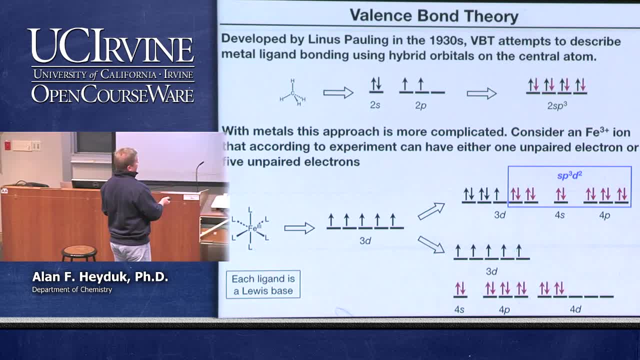 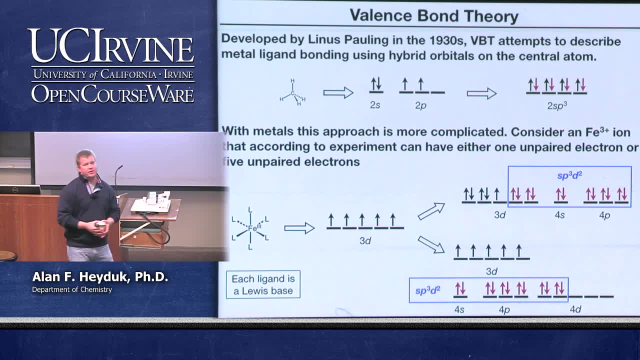 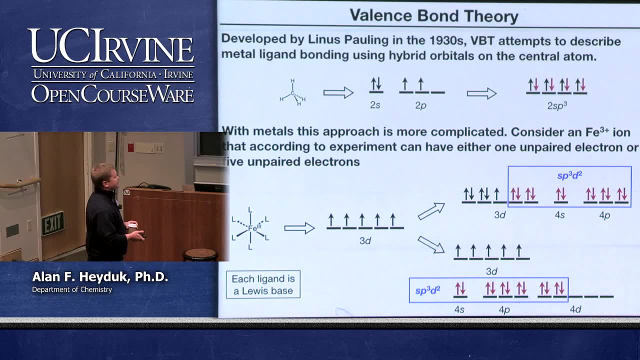 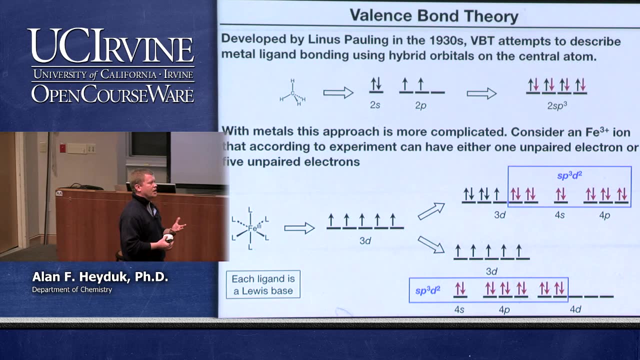 to house the last two pairs of electrons, Ironically, when, if we do this, we end up with the same sort of electron configuration, namely SP3D2 hybridization. Okay, And you may remember that we that that that was talked about a little bit in freshman chemistry. 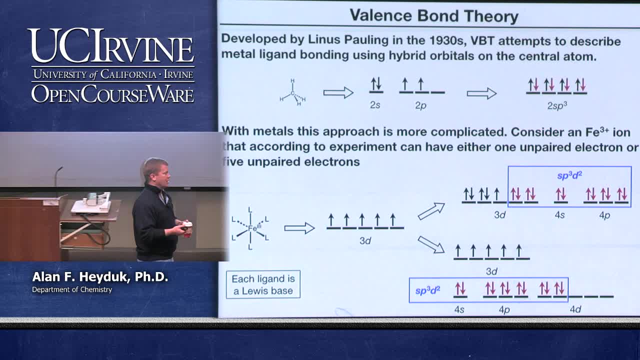 how you would accommodate an octahedral structure. that was that so a six-coordinate metal that was octahedral according to VSEPR, and what hybridization you would need to form those six metal ligand bonds For various reasons. well, this is awful, just just awful. 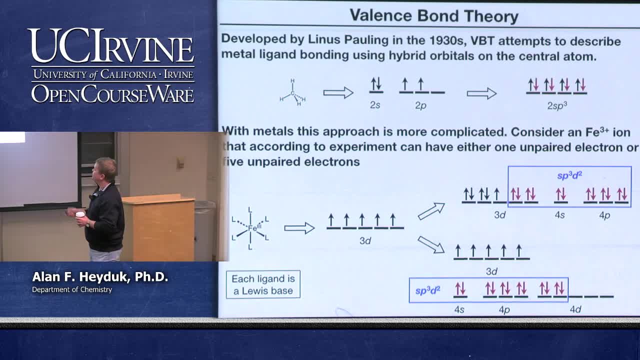 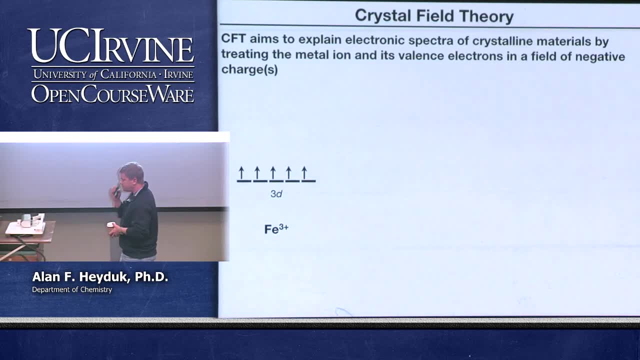 This has problems as well, but it's actually a little bit more accurate. This one is just ugh, Makes me sick to my stomach. So so that approach to to understanding the electronic structure of coordination compounds is a little bit problematic. 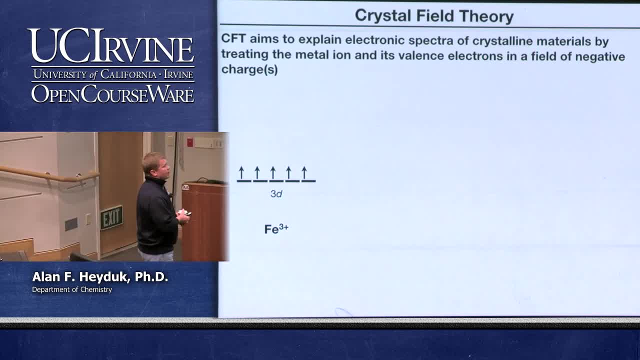 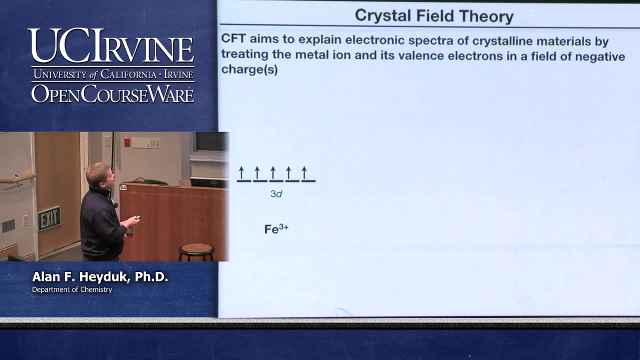 Turns out that, while these molecular methods were being developed, there was also a more physical approach being developed by physicists and spectroscopists who were looking at gemstones and trying to understand their colors, And so what they did is they decided they developed this crystal field theory. 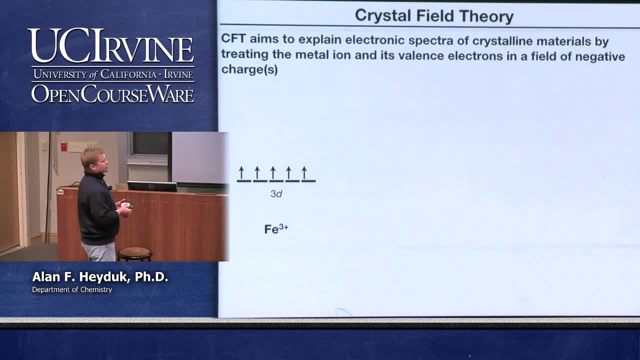 which assumed that coordination complexes were just in a field of negative charge. So if we think about our D5 iron three complex, the way that you would approach it in crystal field theory, this would be just your iron three plus in the gas phase floating around. 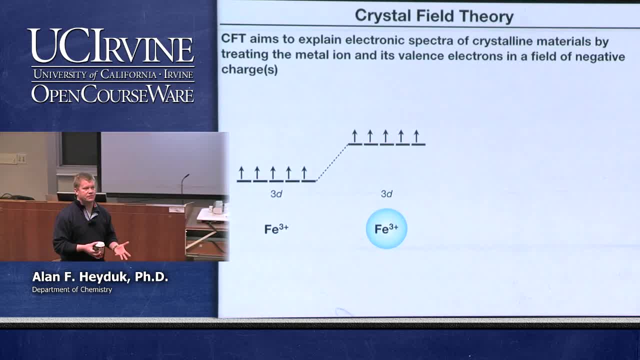 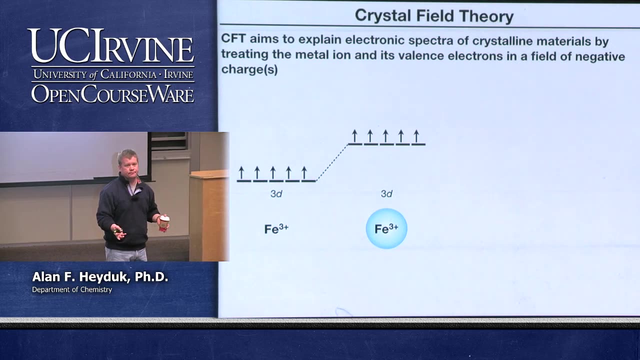 Now, crystal field theory, it's very easy to know, assumes that the ligands are just negative point charges. they generate a negative field around the transition metal ion, and so the first approach is to assume that that electric field is spherical. okay, so the question: what we 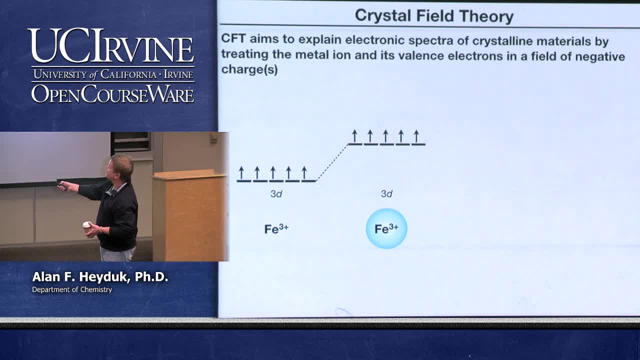 show. here is what happens to the energy of these electrons in the 3d orbitals when we bring in a spherically uniform field of negative charge. well, if the electric field is negatively charged, we know the electrons are negatively charged. there's going to be a repulsive interaction, right? negatives don't like. 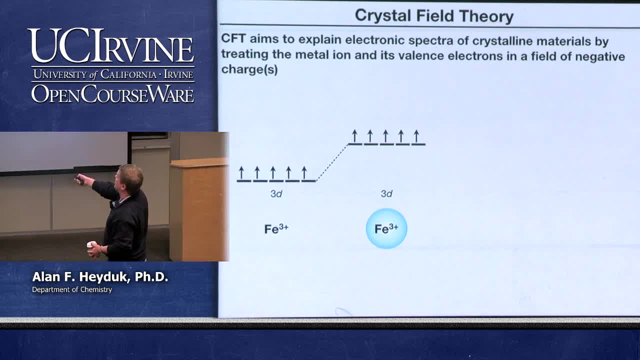 negatives. and so what happens is these d orbitals go up in energy uniformly, because the, the electric field is spherical and uniform all the way around the irons ion. so the next step is to localize this negative field. okay, and so we go from this spherical, even electric field around the, the iron 3 nucleus, to an 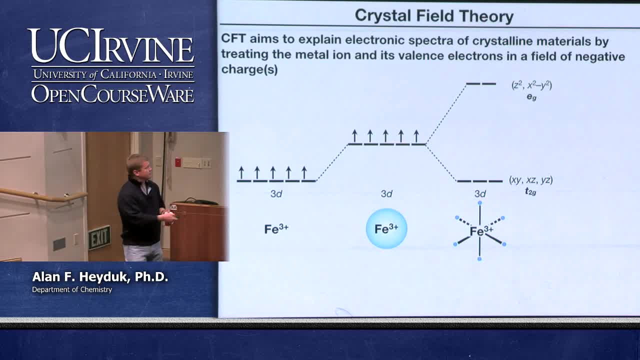 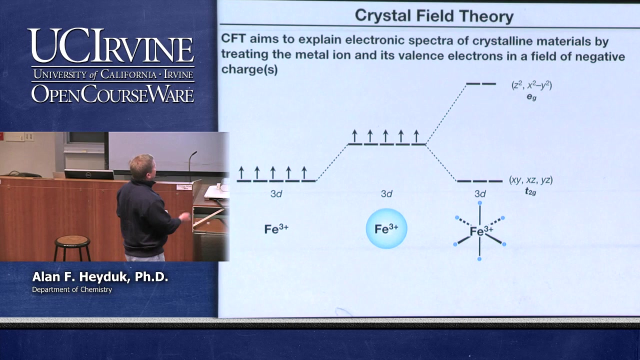 octahedral field. we take the. the total charge is the same as it is in this spherical case, but we just concentrate the electron density into point charges localized along the iron ligand bonds. they define the vertices of the octahedron. okay, and so you can see exactly what happens here. two of the orbitals go up in energy. 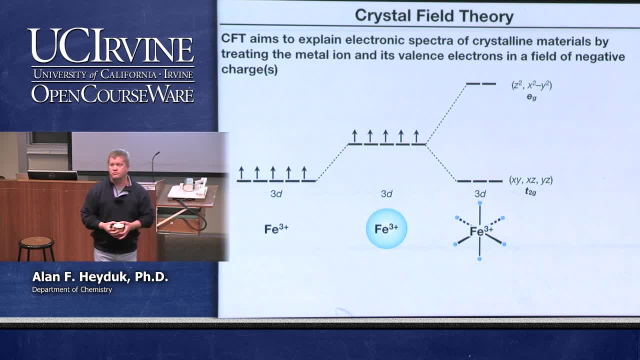 three of the orbitals come back down and if you look at the labels on the on the slide, it should be pretty obvious what's going on. the 2d orbitals that are aligned along the axes are going up in energy because they're pointing directly. 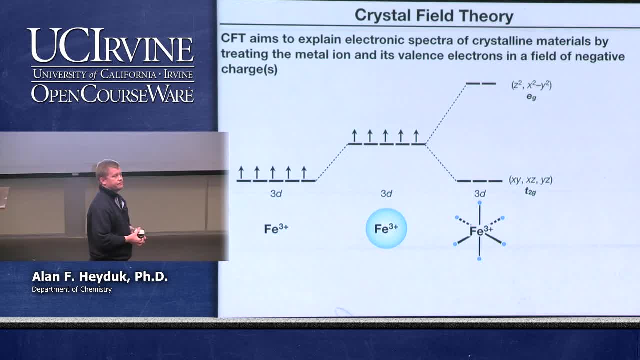 at these negative point charges, the DXY, the DXZ and the DYS. those orbitals are localized in between the metal ligand bonds and so they're not pointing at the negative charges anymore and so Can specify what مع? uir can come back down in energy. 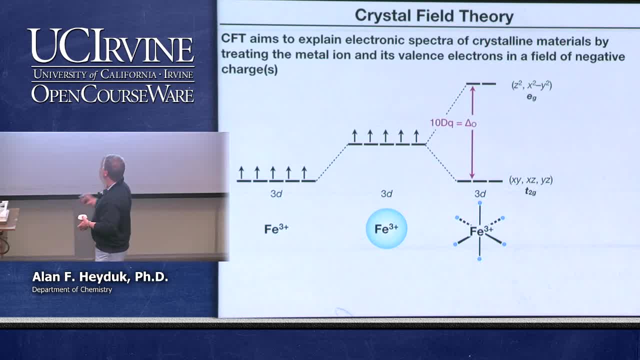 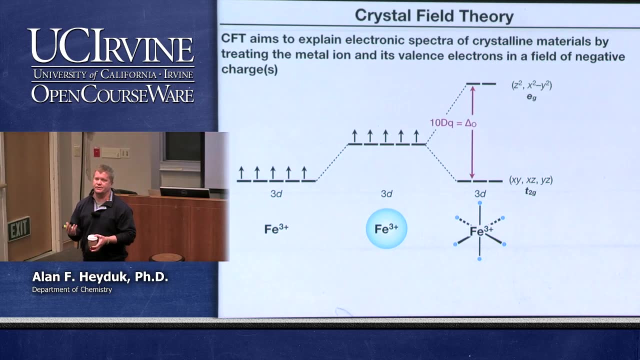 This splitting between the XY, XZ and YZ and the EG orbitals of Z squared and X squared minus Y squared. we call that delta O, the difference in energy for an octahedral crystal field. When you see these, you should know what's coming right. 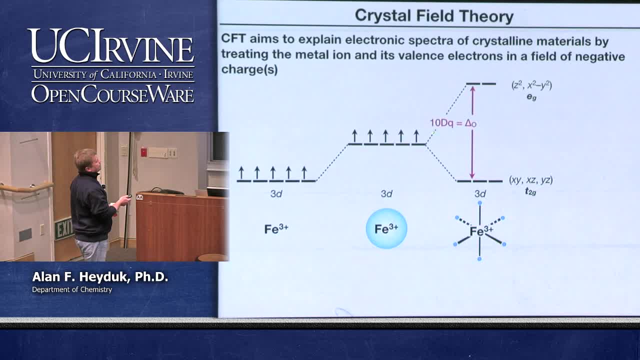 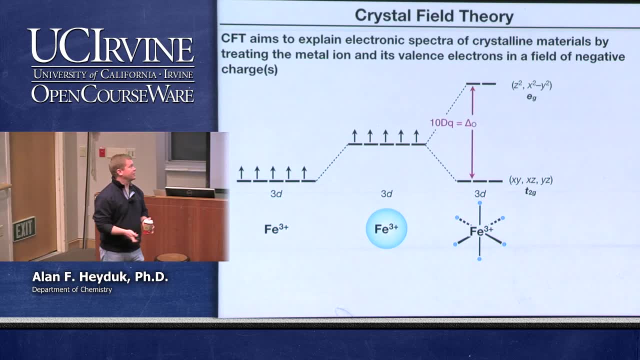 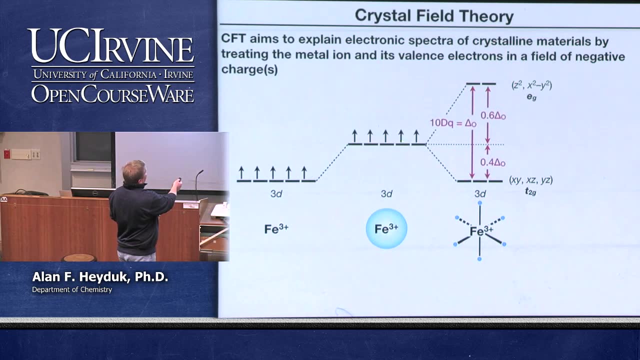 You'll often in old textbooks and papers see 10DQ written instead of delta O. 10DQ is, by definition, delta O. If we take this energy of the free ion in a spherical electric field and measure the amount that EG is destabilized and T2G is stabilized, it turns out that its stabilization is 0.4 delta O, the destabilization is 0.6 delta O and that's done to maintain the symmetry, or the, if you want to think about it, the center of energy. you know, like the center of mass, but the center of energy. 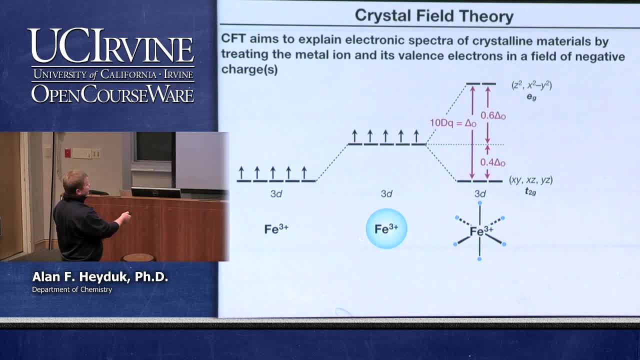 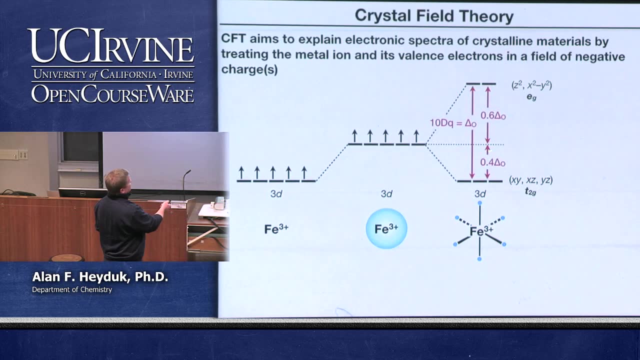 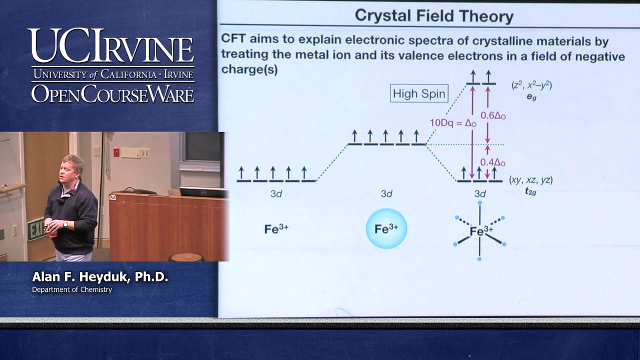 And that's because the intensity of the electric field doesn't change from here to here, so the total destabilization has to remain the same. If these two orbitals go up by 0.6,, then three orbitals come down by 0.4.. 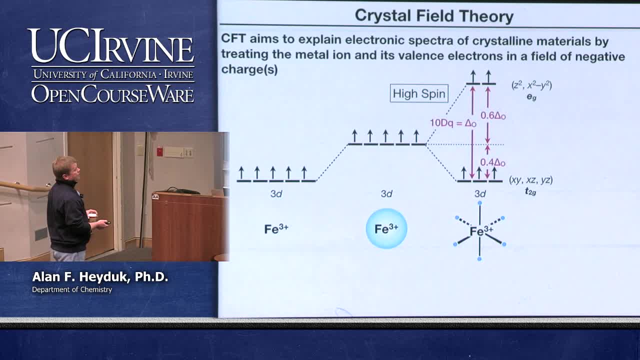 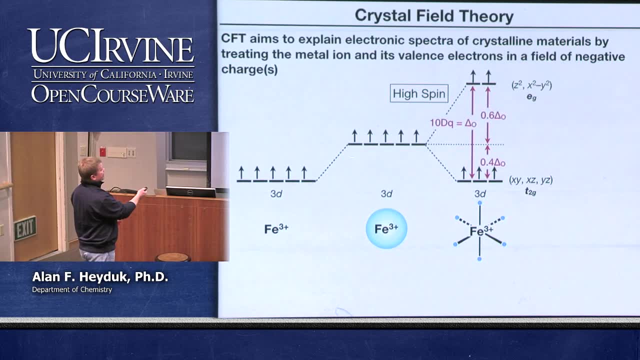 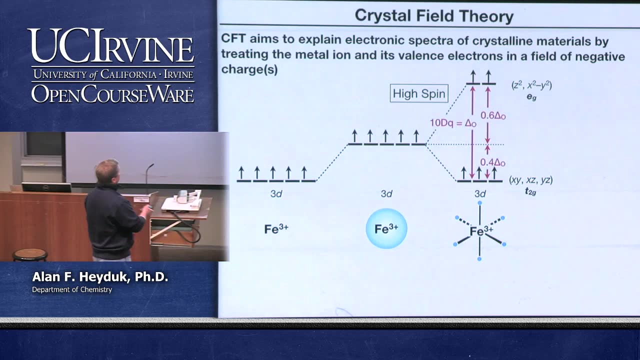 In an iron three plus compound, we end up with two spin options. Okay, The first one follows straight from what we would learn, what we learned in freshmen chemistry, where we put all the electrons in spin up and spread them out over the five equivalent. 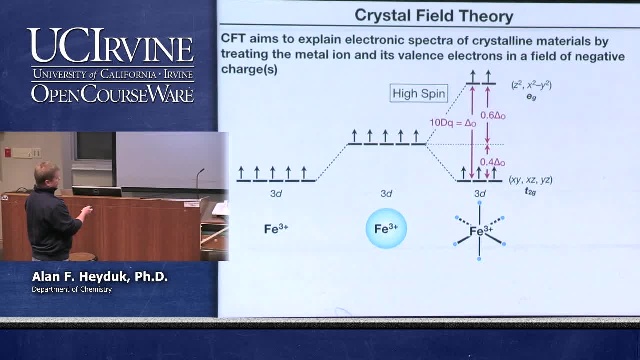 orbitals. We call this the high spin case. We put three electrons in T2G, two electrons in EG. everything's pointing up. The other alternative is what you might think of as the more organic approach. Okay, Okay, Okay. Okay, And that's the low spin electron configuration, where all five electrons go into the T2G. Of course, that means that two of the electrons have to have a down pointing spin, And so it's called the low spin configuration, because the net spin of this iron complex is only 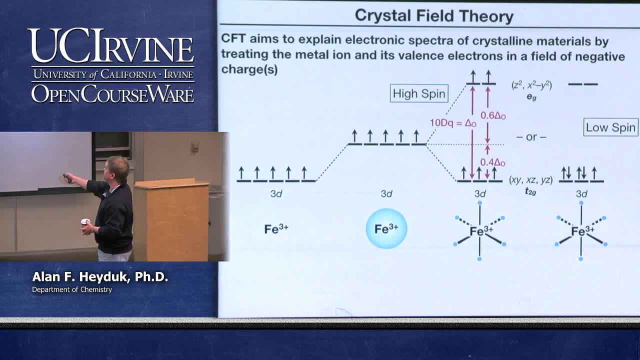 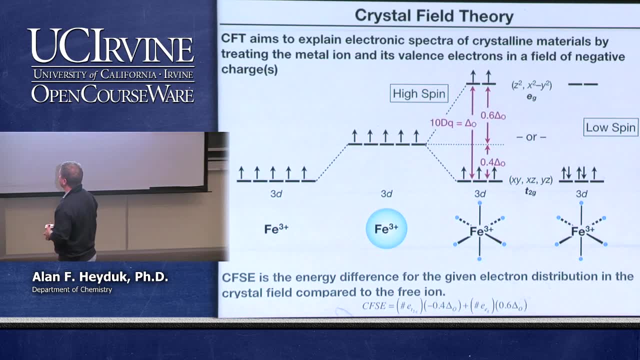 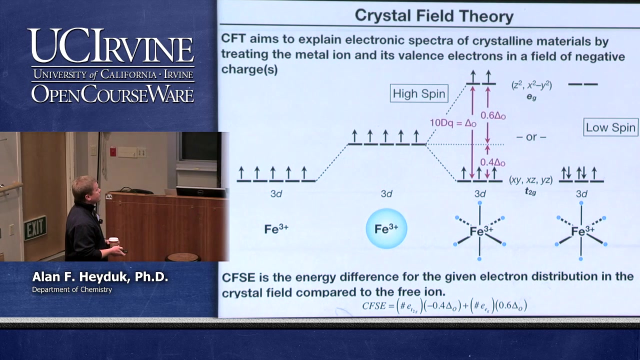 to have one unpaired electron pointing up as opposed to five unpaired electrons all pointing up in the high spin configuration. So one of the things that crystal field theory allows you to do is calculate the net stabilization of a given electron configuration compared to this free ion form. 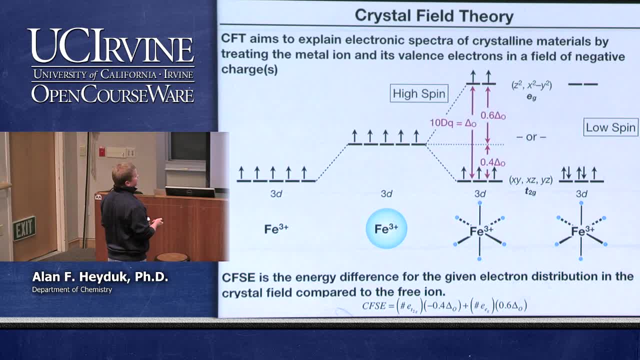 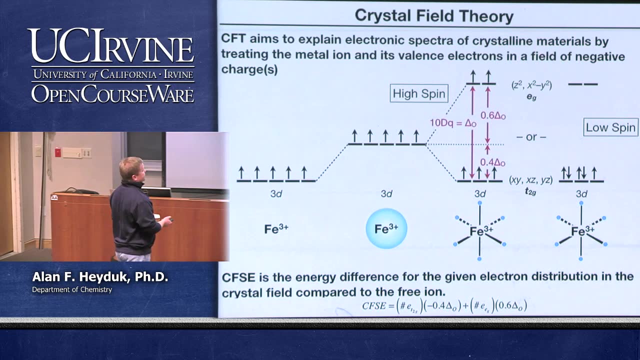 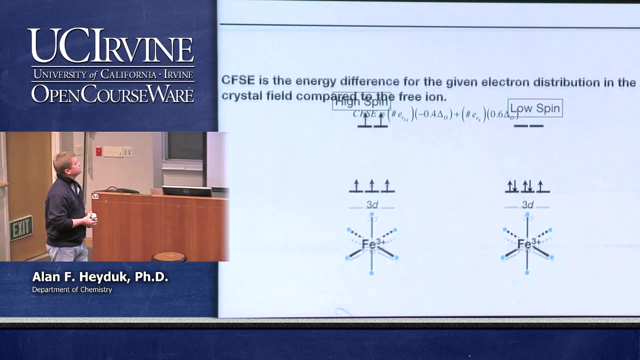 And so the crystal field stabilization energy is defined as the number of electrons in the T2G orbital times minus 0.4 delta O, And we add to that the number of electrons in the EG orbital times positive 0.6 delta O. So we can look. 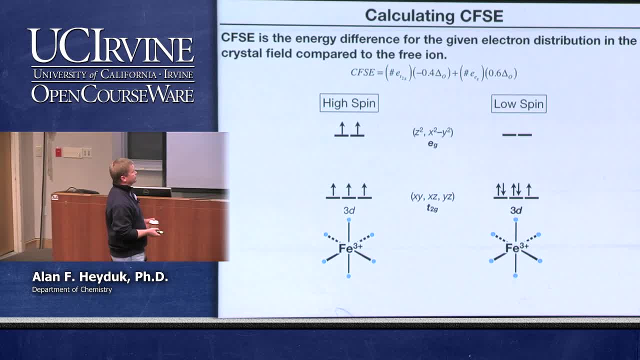 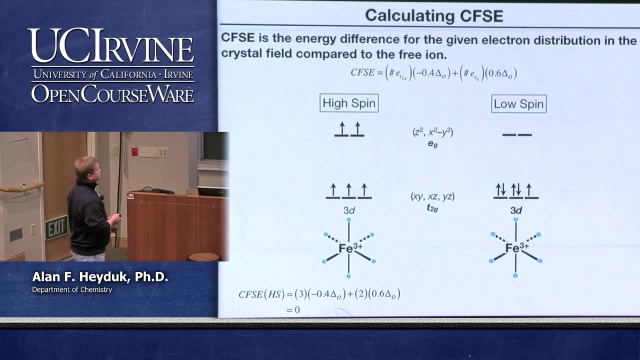 at our two possible electron configurations- The high spin case And the low spin case, And we can use the crystal field stabilization energy to start asking which is more favorable. And so, for the high spin case, we have three electrons in T2G. 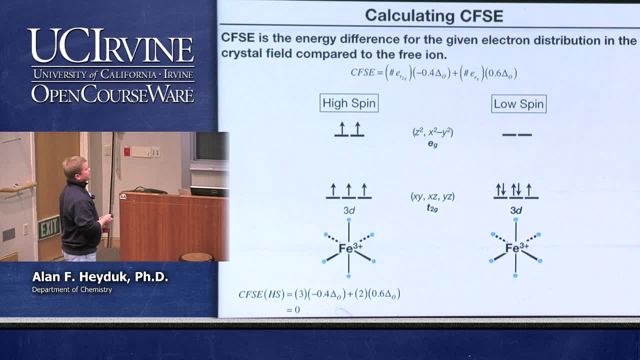 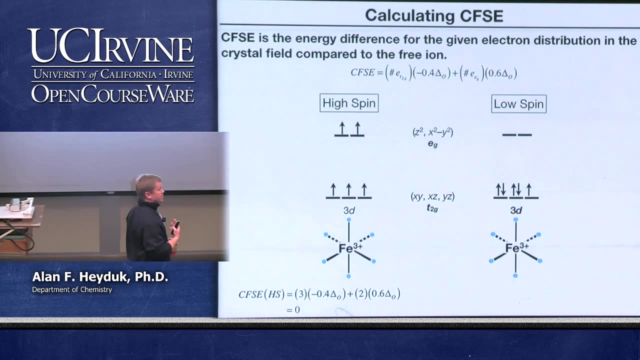 two electrons in EG. When you calculate the crystal field stabilization energy, you come up with zero. So this electron configuration has no advantage over a purely spherical electric field. That's the way that you can interpret a crystal field stabilization energy of zero. 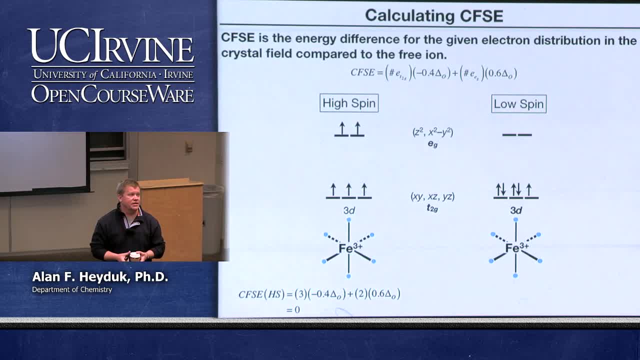 Localizing the electric field on the vertices of an octahedron did nothing to stabilize the ion relative to a perfectly spherical electric field. On the other hand, for the high spin configuration we have five electrons. All of them are in T2G, zero in EG. 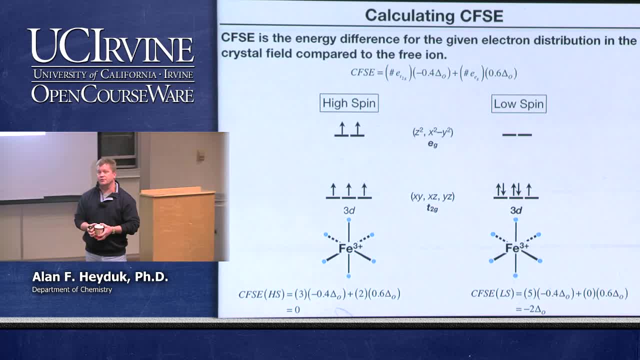 And so when we calculate the crystal field stabilization energy for the low spin configuration, we calculate that the energy is minus 2 delta O. So if delta O is this splitting the crystal field stabilization energy is negative, It's going to be a negative number. 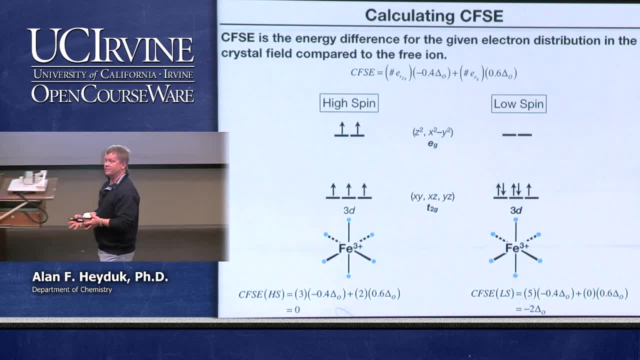 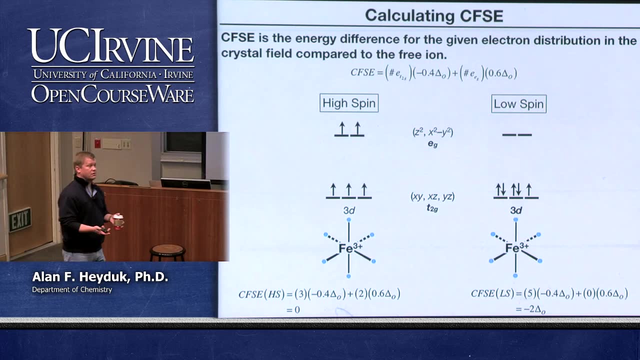 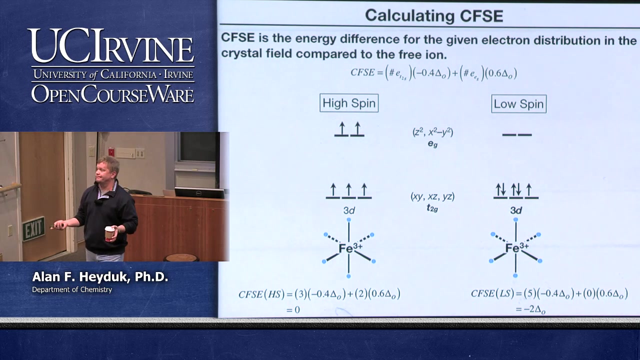 We know that, based on our energy conventions, negative numbers tend to be lower energy species than positive, So clearly the low spin configuration should be favored, according to the crystal field theory. Now what's the catch? Who knows what the catch is? Yeah, It costs energy to take two electrons. 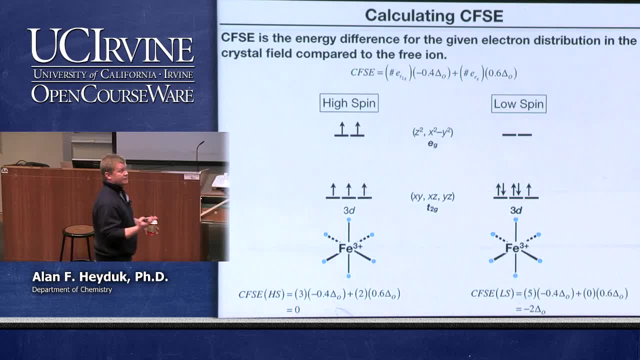 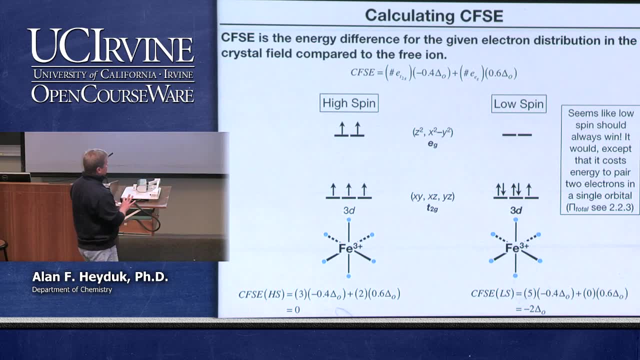 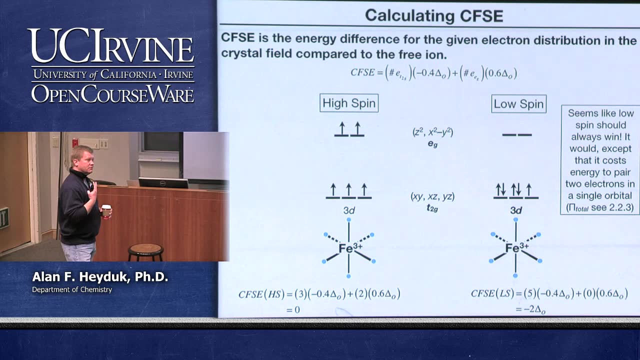 and put them in one orbital, Because negative charges repel each other. So according to crystal field theory, you might predict, at least at this very preliminary stage, that you would always favor the low spin configuration. But because it costs energy to put two electrons 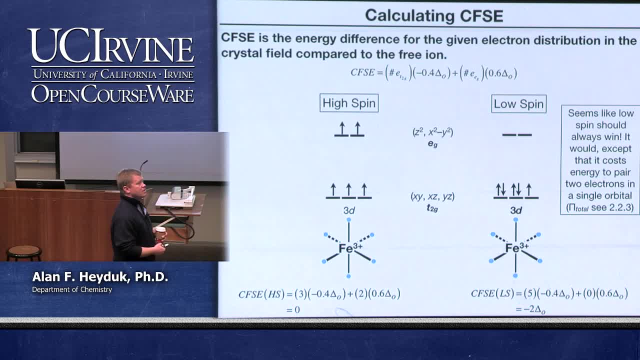 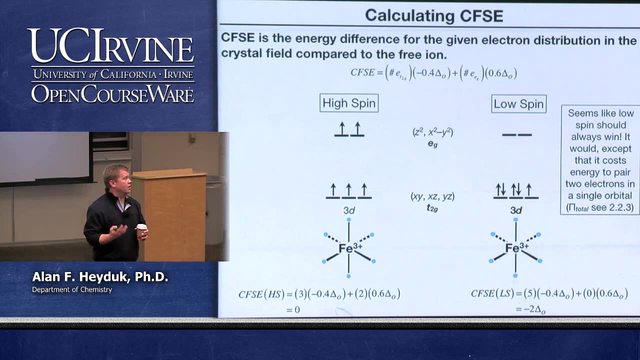 in the same region of space, they repel each other. you have to balance that out with the electron pairing energy. We'll talk about that in a few slides. But in short, the smaller the orbital, the more pairing energy there will be. 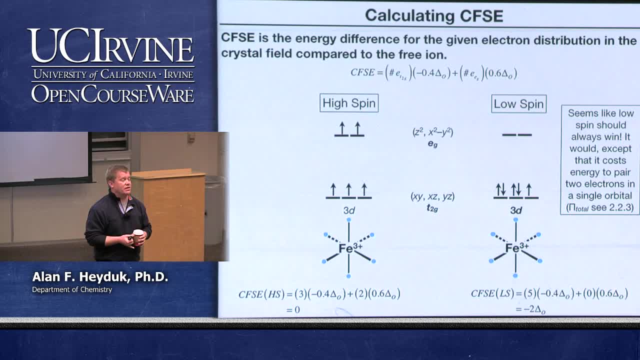 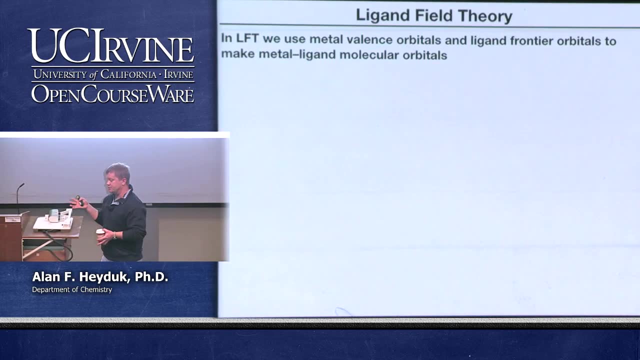 the more difficult it will be to put two electrons in it and the more likely for a high spin configuration. OK, So crystal field theory was a pretty good start to understanding the electronic structure of transition metal complexes. We just looked at it in a very preliminary way. 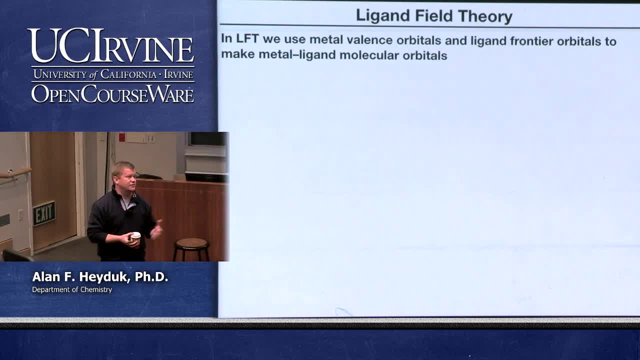 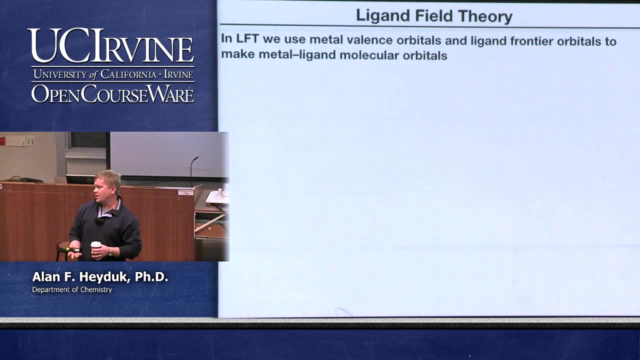 But it does a pretty good job with a variety of ions and different electron configurations. But as a chemist- OK, remember, it was developed by physicists. Come on, As a chemist, there are some things that should bother you. OK, We're approximate. the whole theory is built. 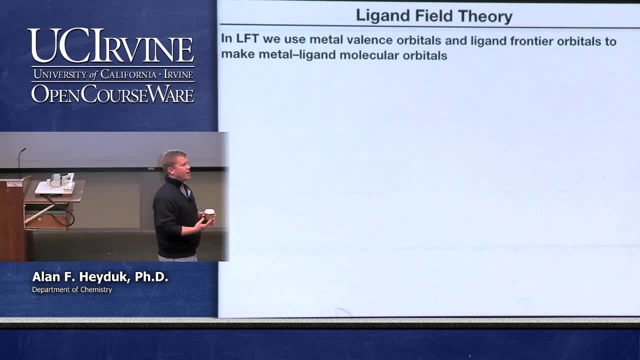 on this idea that a ligand can be approximated as a negative point charge. OK, So in other words, what they're saying is the interaction between the metal ion and the ligand is purely electrostatic. OK, That's probably not such a bad thing if you're looking. 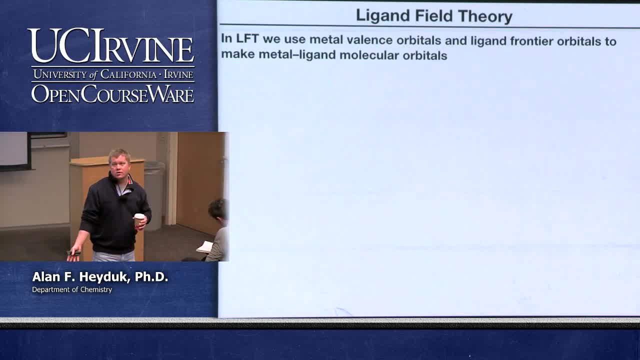 at titanium oxide or obviously something like potassium chloride, Electrostatic, Electrostatic interactions are going to dominate. But what if you're looking at an organometallic complex where you have a metal-carbon bond That somehow seems maybe problematic, right? 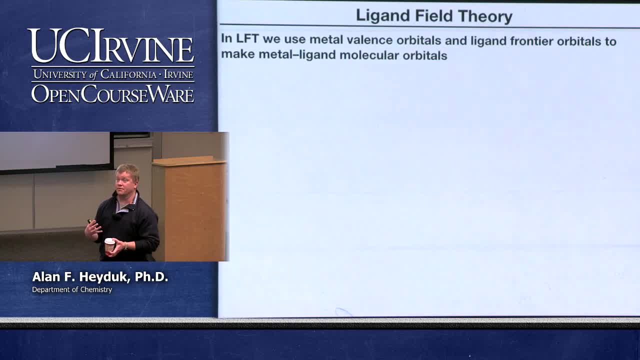 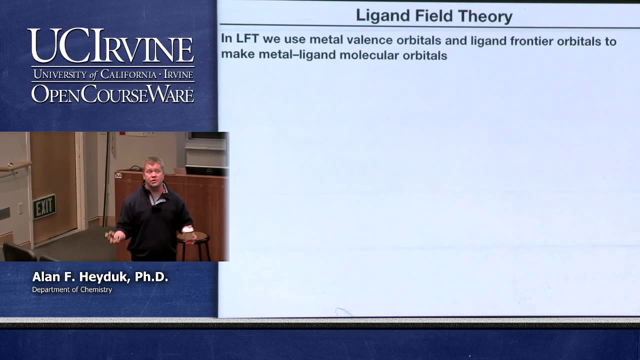 We know that in organic compounds there's something more to it than electrostatic interactions: There's covalency. Crystal field theory does not allow any for any covalency. OK, That's a huge, huge shortcoming of the model. 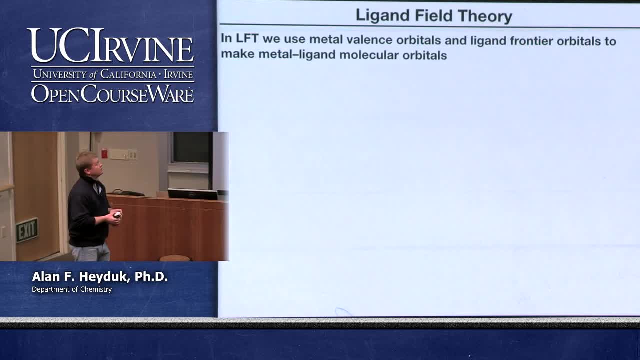 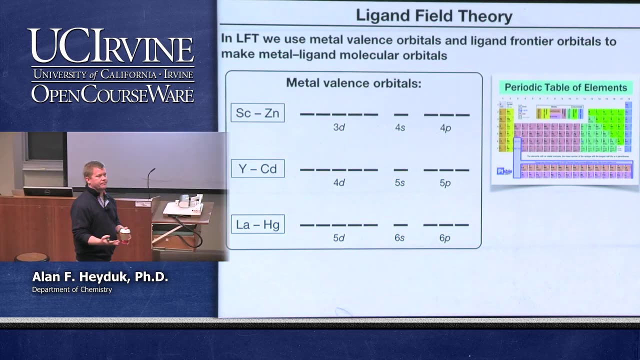 And so probably about 60 years ago now. 60,, 70 years ago, ligand field theory came about, And what it really seeks to do is combine crystal field theory with molecular orbital theory so that you can get both the electrostatic and the molecular orbital theory. 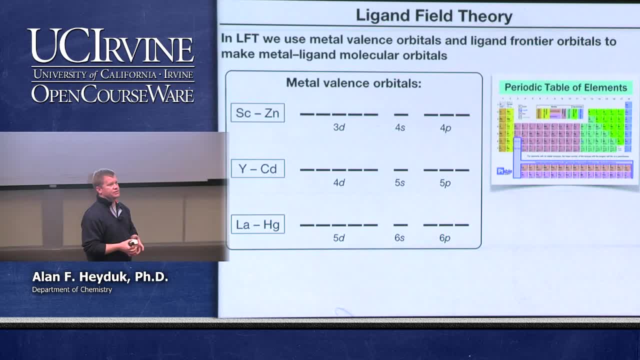 So that the trilogy has the same amount of space and just has a different type of space than the molecular orbital theory does. and it can be done for emissive and ол-static-type interactions described by crystal field theory, including high spin, low spin-type designations. 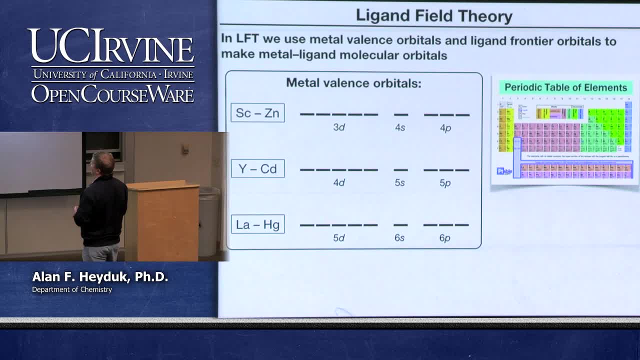 along with covalency. that's described very well by molecular orbital theory, And so for ligand field theory, we have to understand what the frontier orbit atomic orbitals are. for the transition metals, For the first row, we have a free radical right. 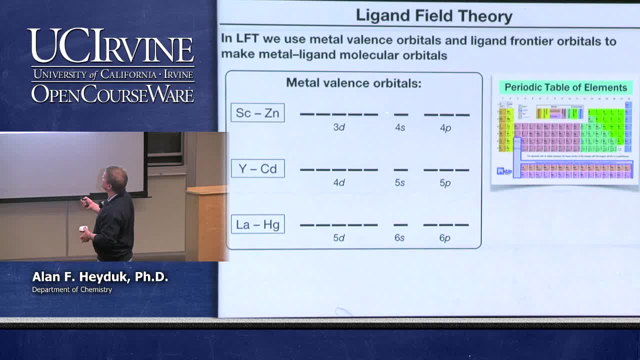 and we have a free electron For the first row of the transition metal series. it's going to be the 3D orbitals, the 4S and the 4P As we drop down. we can just add one to each principal quantum number. 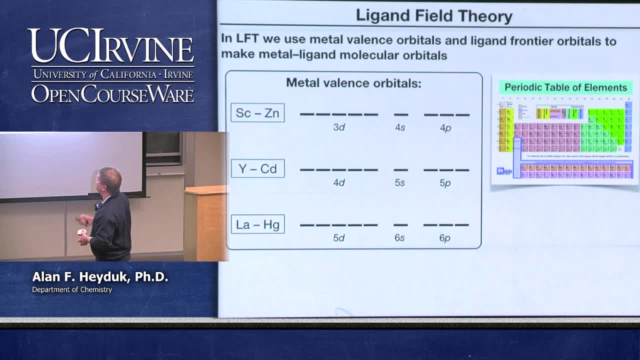 So for yttrium through cadmium- 4D, 5S and 5P, and lanthanum through mercury- 5D, 6S and 6P. Now I'm going to put a. there's a huge footnote here. 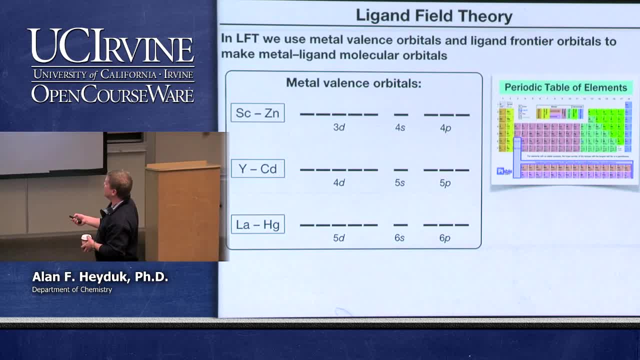 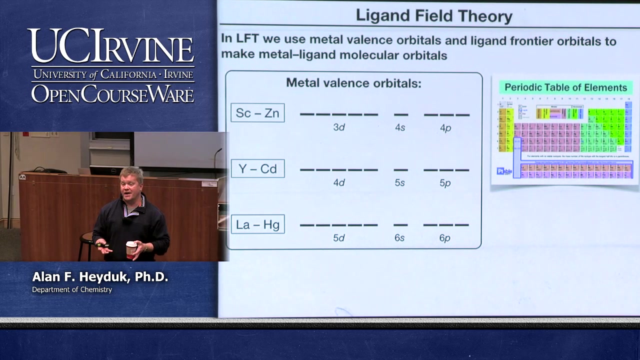 Even though I went lanthanum through mercury and yttrium through cadmium, there's this whole block of elements that drop down here, the lanthanides and the actinides. It turns out that they're very- they're kind of special in that the introduction of F orbitals and the increase in Z effective, the effective nuclear charge associated with the F orbitals. 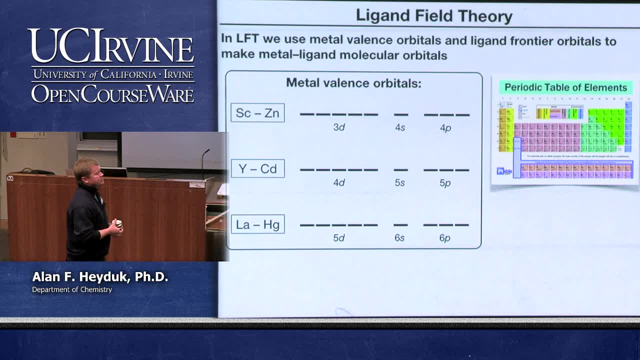 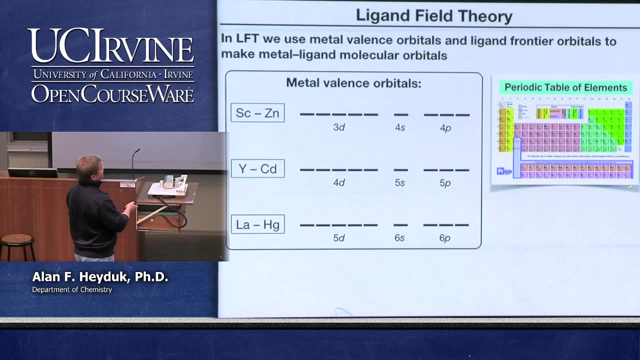 results In these lanthanides and actinides, the bonding being dominated by electrostatic interactions. Covalency in lanthanide and actinide complexes is minor. Okay, And so it turns out that for trying to understand the complexes, or the electronic structure of complexes of these metals, 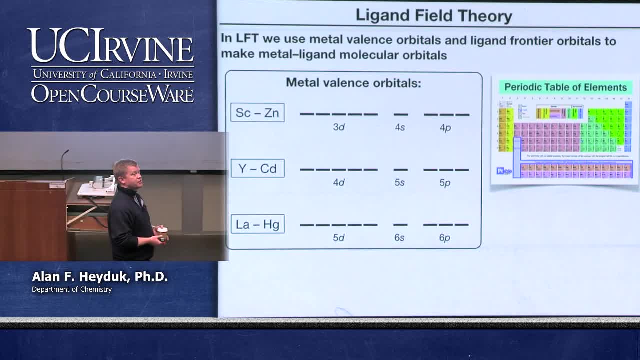 really all you need to use is crystal field theory to a first approximation and it will get you pretty darn close, Because the F orbitals generally don't split and they don't participate in bonding and they typically all stay at about the same energy. 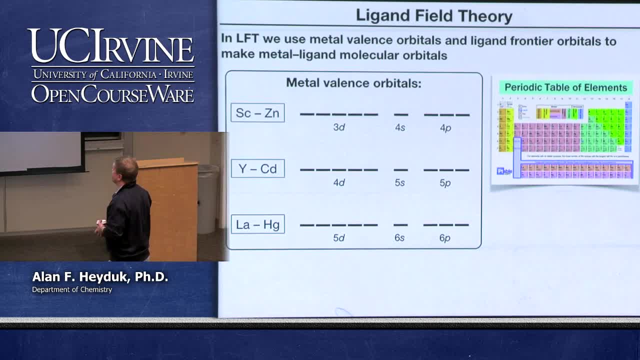 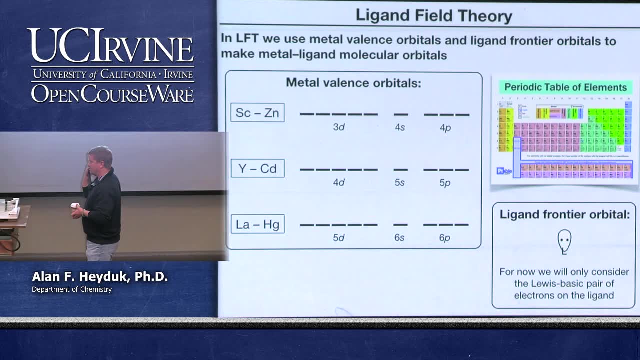 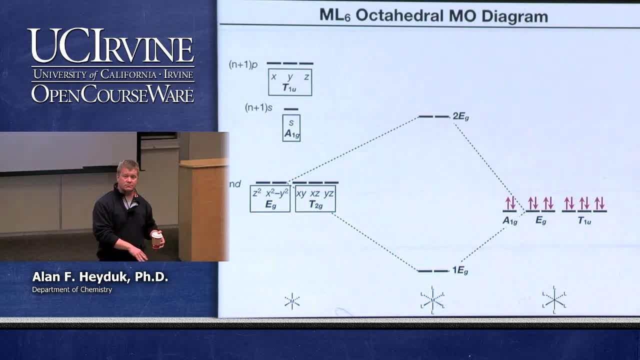 Well, for now we're going to start by just assuming a pair of electrons that point to the electron structure of a coordination complex. it You make a bonding orbital and an anti-bonding orbital. The next pair that we see is A1G. 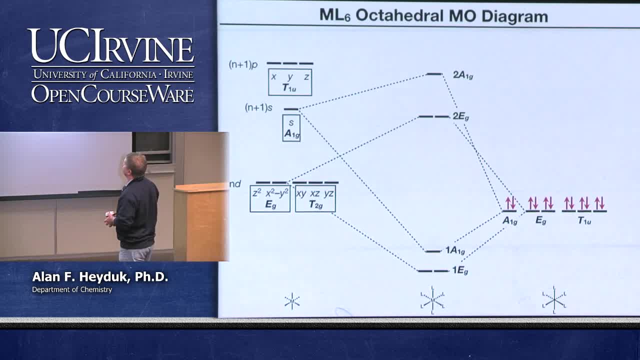 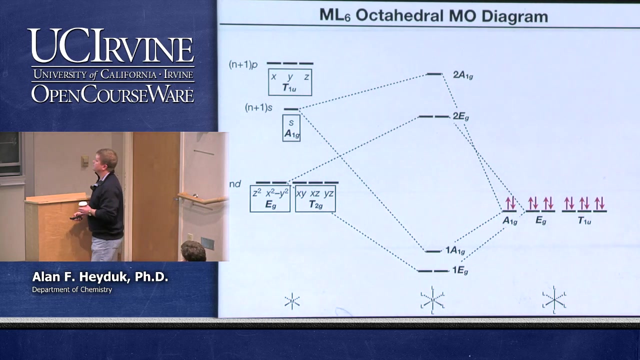 the S orbital on the metal and this A1G symmetry orbital on the ligands. We make a bonding combination and an anti-bonding combination. Finally, the metal has the T1U symmetry P orbitals and the ligands have a T1U symmetry set of Lewis basic electron pairs We make 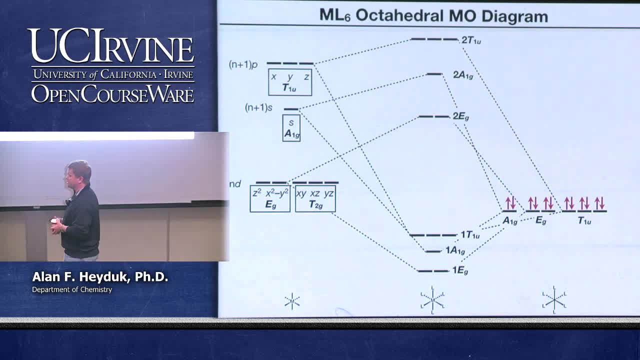 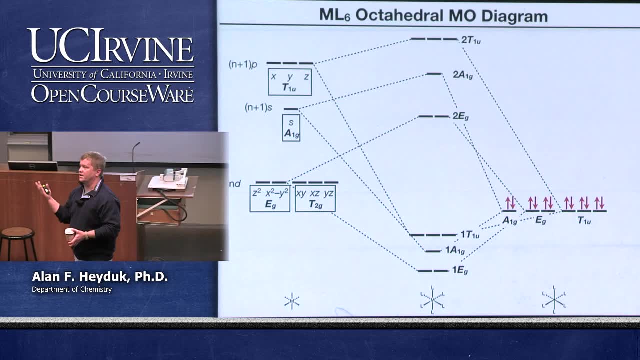 the bonding combination, we make the anti-bonding combination. Now you're going to. now you're going to. Now. you're probably asked: well, how do I know how far down to stabilize the bonding combinations and how far up to push the anti-bonding combinations? 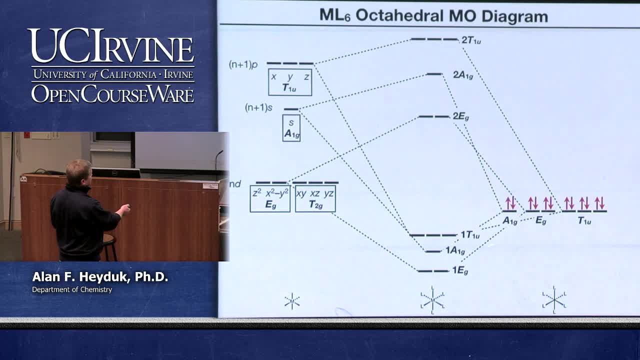 Why did I drop the EG orbital way down here, but this T1U I didn't drop very far. Why would I do that? Because the other side is higher. Remember, we also learned that the strength of an interaction is inversely proportional to the separation. 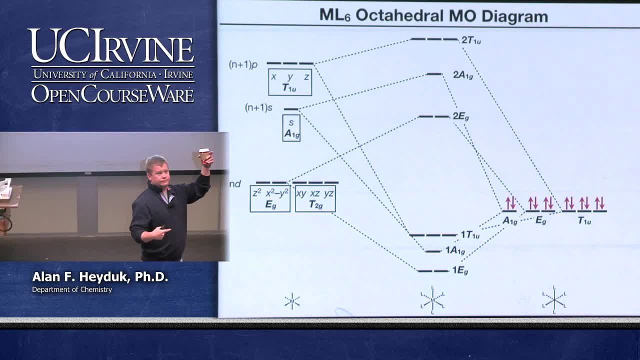 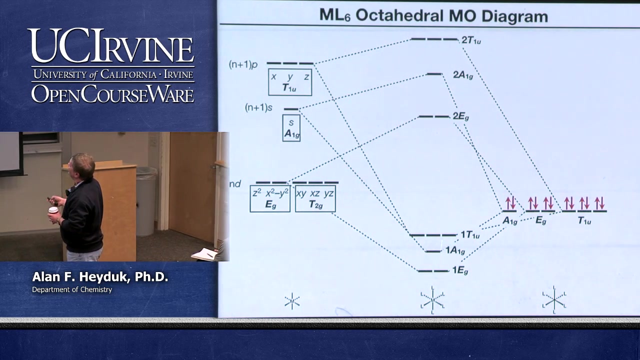 in energy between the two fragments. This is my favorite analogy. It's the high-energy cheerleader and the low-energy chemistry major. They just don't interact. Okay, It's an approximation that will get you in the ballpark. Now you'll notice that we've used up all three representations. 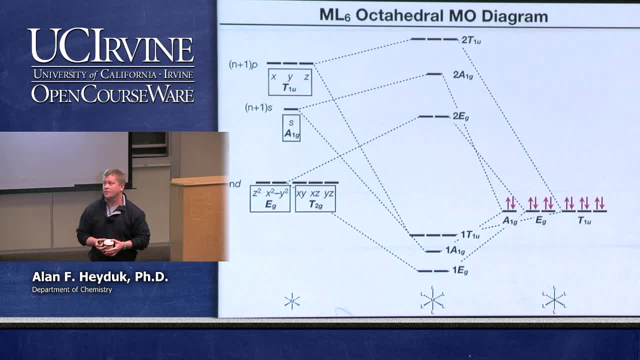 of Lewis basic electron pairs on the ligands We still have one left over, one set of orbitals left over on the metal. the T2G That just comes across unperturbed doesn't change because there's nothing on the ligands for it to interact with. 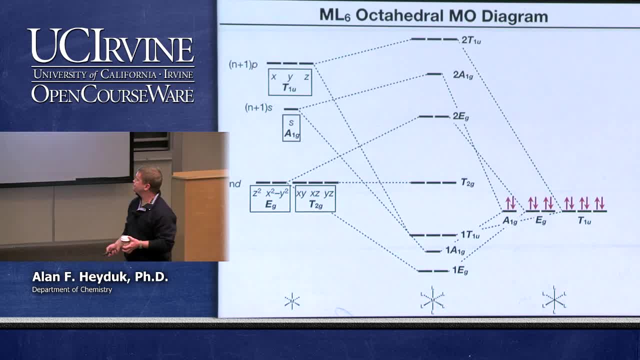 Those are non-bonding orbitals in this problem. We take our 12 electrons that our Lewis basic ligands brought in and they go in the lowest six energy orbitals on the diagram, Those six orbitals, the reason we brought them down in energy. 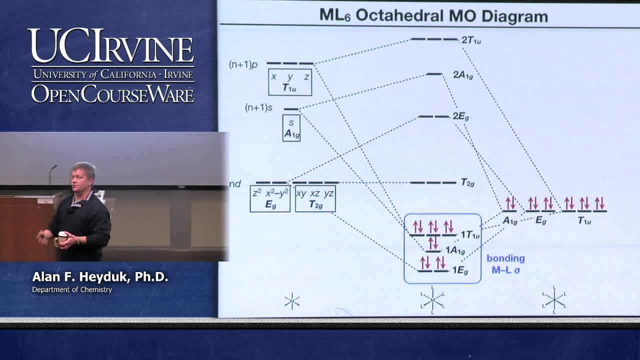 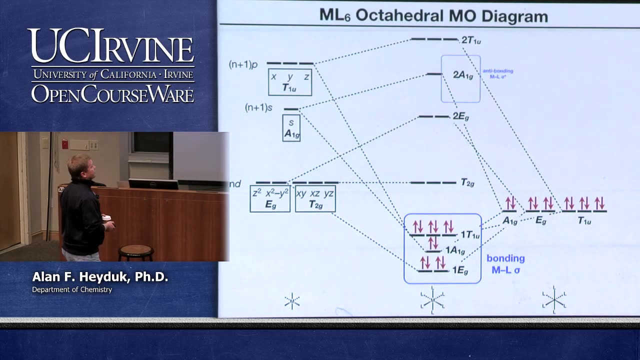 is because they're bonding orbitals. Those are the six orbitals that we call the metal ligand sigma bonds. That's what holds it together. If we have six metal ligand sigma bonds, we darn well better have six metal ligand sigma star. 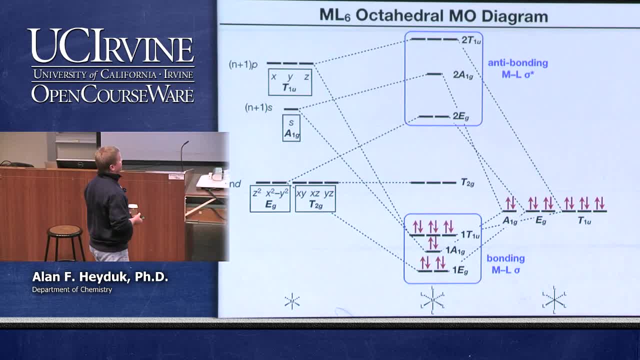 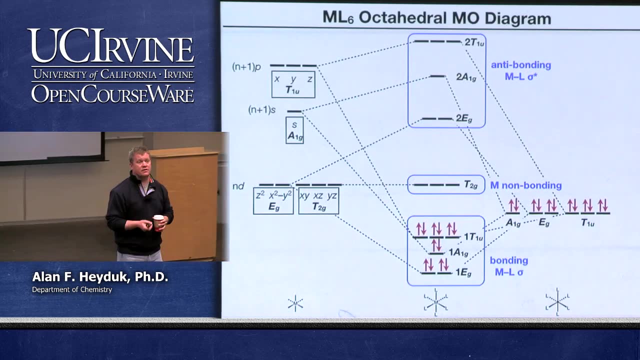 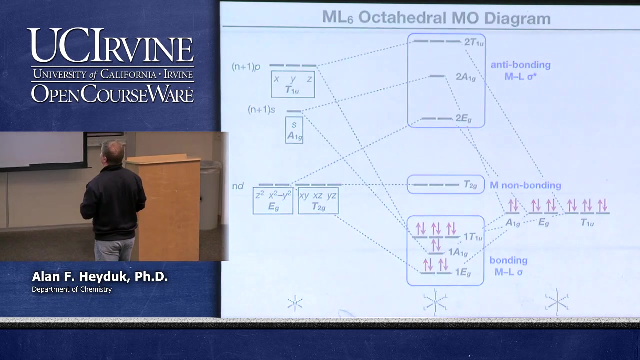 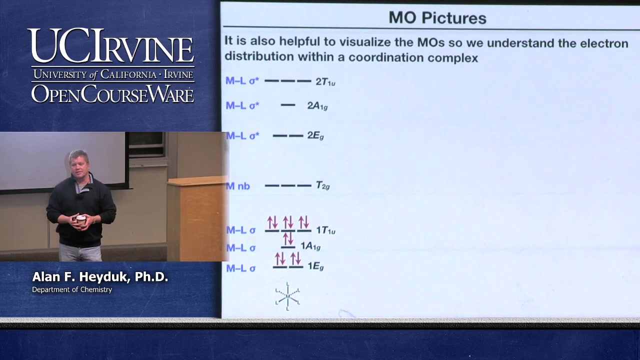 Those are the out-of-phase combination That T2G set purely on the metal, no contribution from the ligand. therefore they look just like metal ligand D orbitals and they're non-bonding. So I talk a good game when I talk about secular determinants. 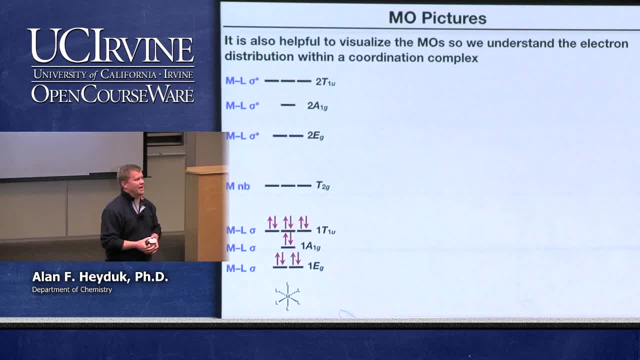 and block, diagonalizing and wave functions and all this. I'm not a math guy, I'm a cartoonist, I'm a cartoon guy, And so for me it's always really, really helpful to see pictures of what these orbitals look like- the cartoons. 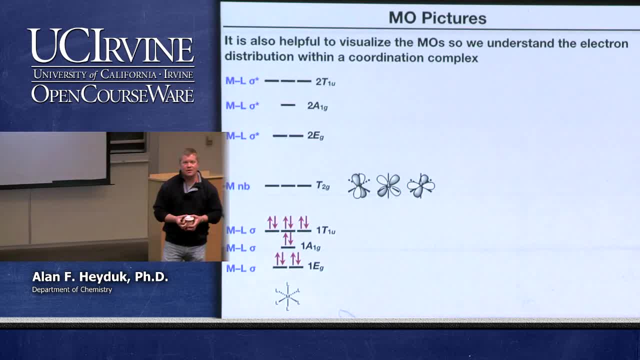 So we can go through. hey, those are the easy ones. There's those T2G orbitals that we said were non-bonding. They're the metal DXZYZ and XY orbital. piece of cake, What do the rest of these orbitals look like? 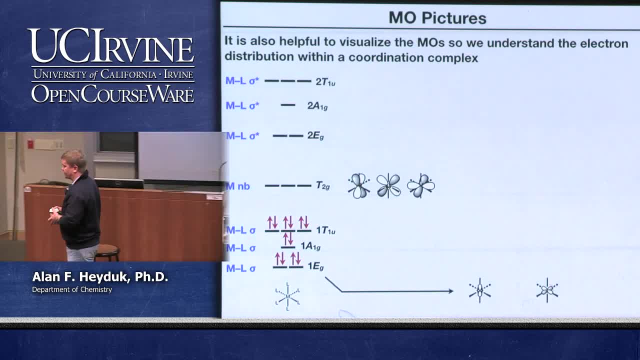 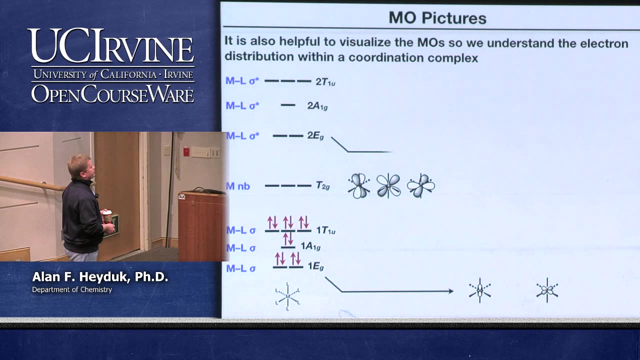 Well, we'll start with the EG, And so we know that the EG component from the metal is DZ squared and DX squared minus Y squared, And so that's going to appear here in one EG and what I've labeled two EG. 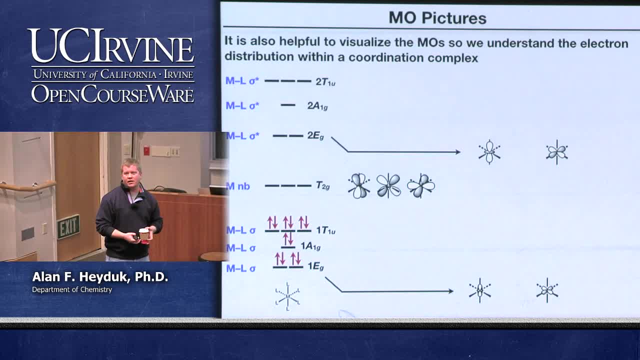 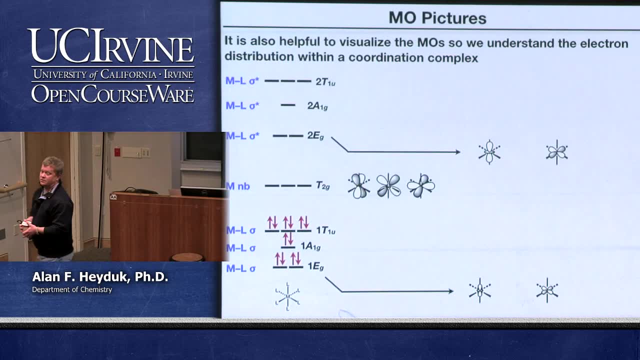 That coefficient is just telling you. you know, this is the first EG orbital and that's the second EG orbital. You can call them A and B if you want. Barney and Fred, I don't really care. Laverne and Shirley, it's okay. 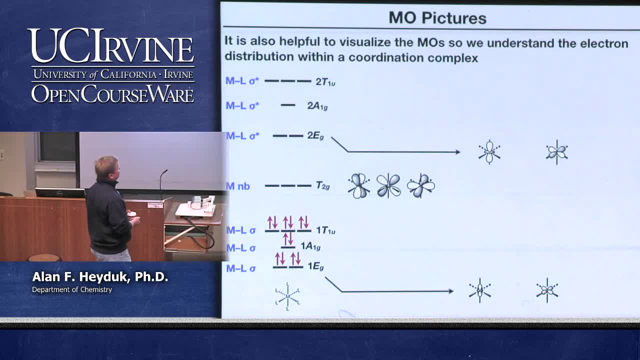 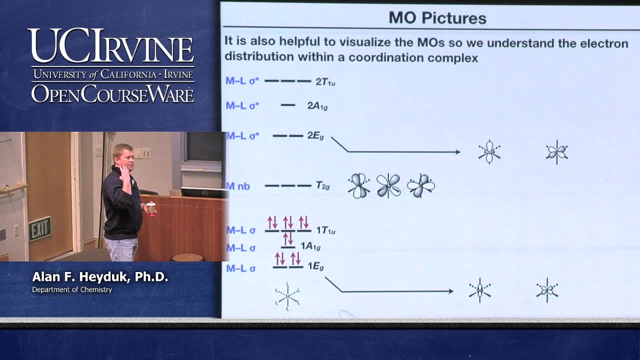 I'm good with all those One and two just fits on the slide better. So the EG contribution from the metal is going to be DZ squared and DX squared, minus Y squared in both cases, And we can actually use the picture of the metal orbital. 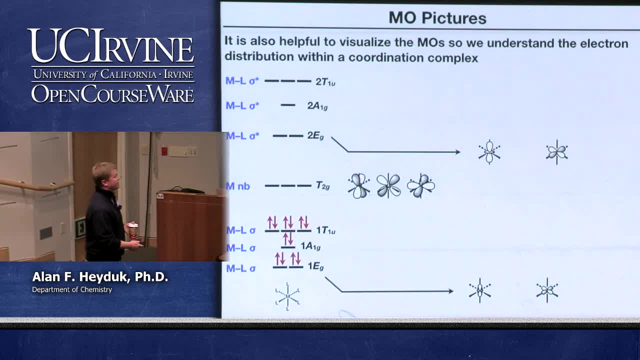 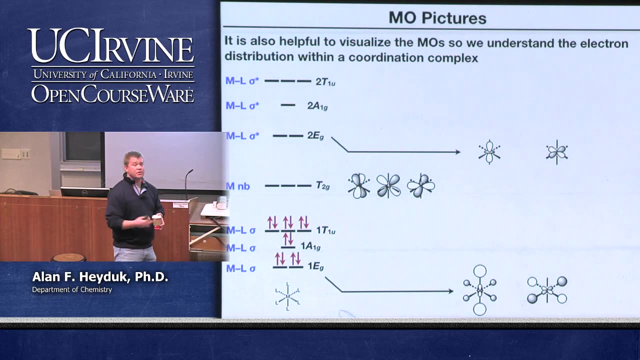 to predict what the length is. So you can see what the ligand orbital looks like or the ligand contribution looks like. In the bonding case, we're going to have in-phase contributions in every direction. You can also use the projection operator. 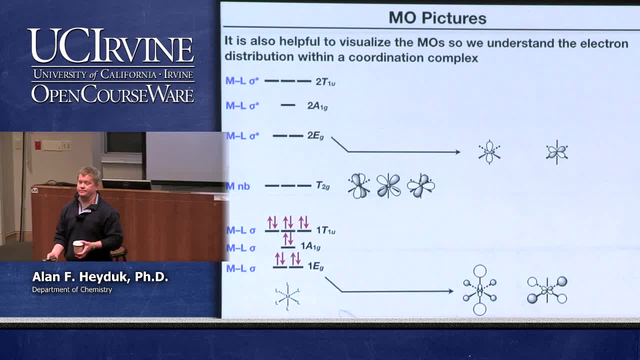 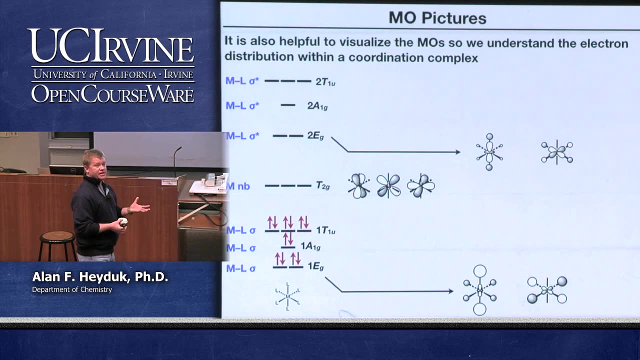 to calculate what the ligand contribution looks like. Okay, After you've done it enough times and you've gotten enough practice, you're going to realize that you can just predict Real quickly what it looks like. The shape is going to be the same in the bonding. 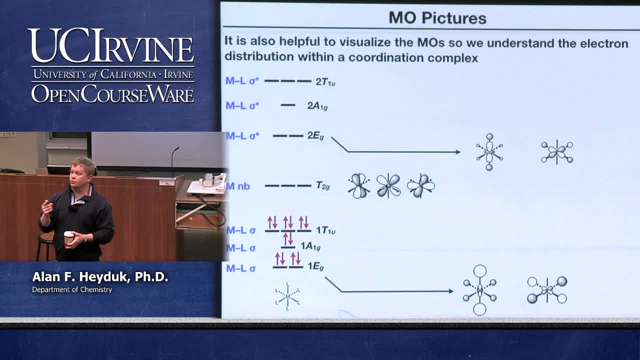 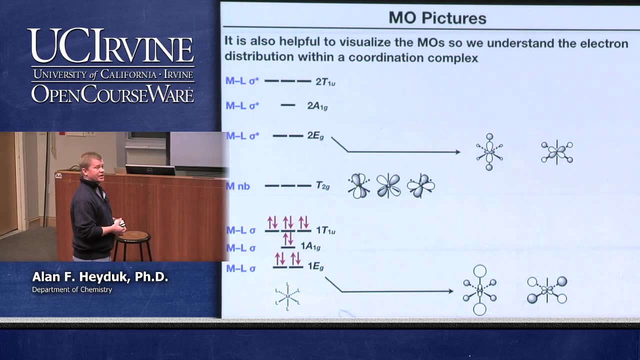 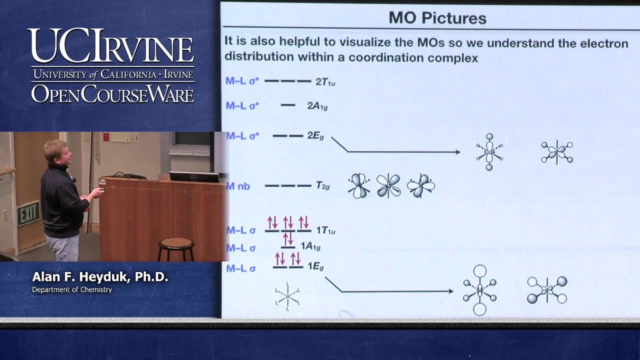 in the anti-bonding orbital. but the relative contribution is going to be different. You'll notice down here. in the bonding combination we have a relatively big contribution from the ligand and a relatively small contribution from the metal. Okay, In the anti-bonding combination we have a big contribution. 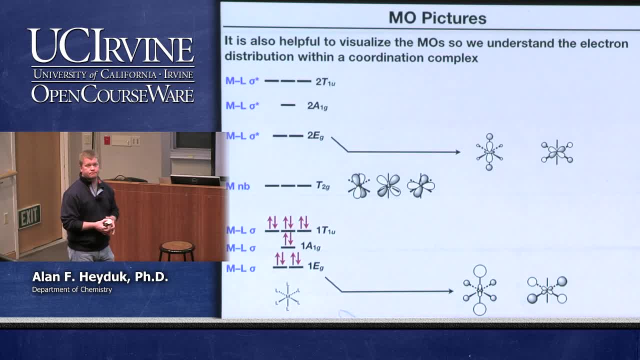 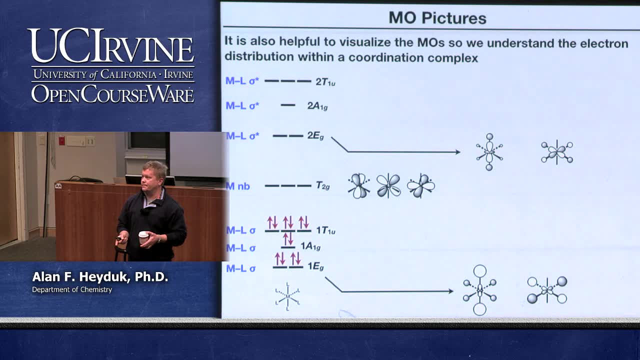 from the metal and a small contribution from the ligand. Remember, these are Lewis acid-Lewis base interactions. Okay, We're starting with a pair of electrons on a ligand, on a Lewis basic ligand, the HOMO of the ligand. 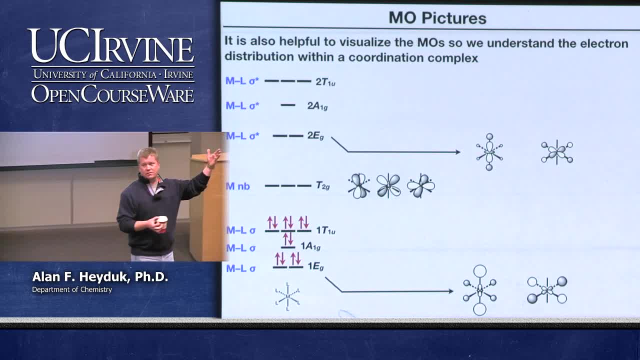 and we're starting with the LUMO of the metal, an empty Lewis acidic orbital. Okay, We're starting with an asymmetric energy. The ligand orbital is lower than the metal, and so the bonding orbital will be localized on the ligand. 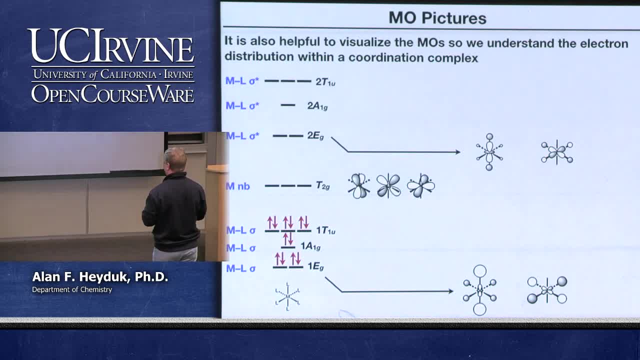 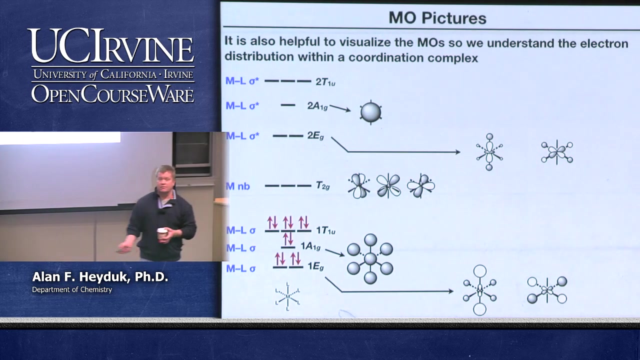 The anti-bonding orbital will be localized on the metal. We can repeat this process for the rest of the orbital combinations. The A1G contribution from the metal is the S orbital, both to the bonding and anti-bonding. No surprise, the ligand contribution. 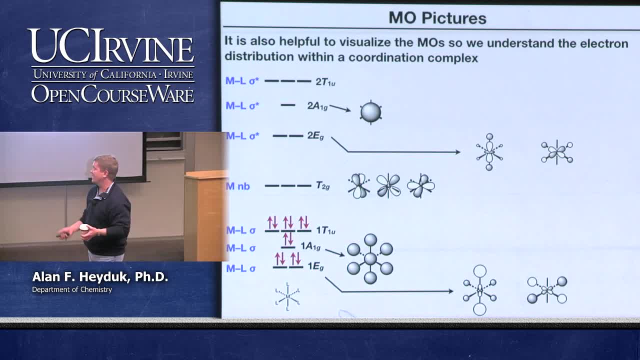 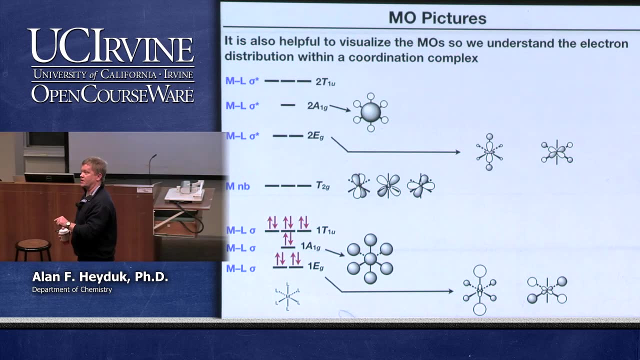 to the A1G is going to be completely symmetric. Everything in phase dance party, because everybody's happy. The anti-bonding combination, all of the ligand contributions have the same phase, But it's opposite of the metal contribution. That orbital, the anti-bonding orbital, is also localized. 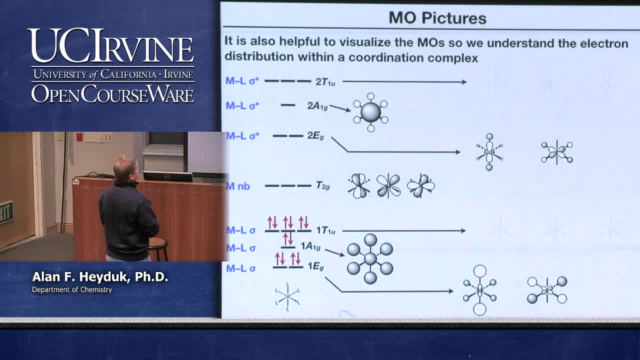 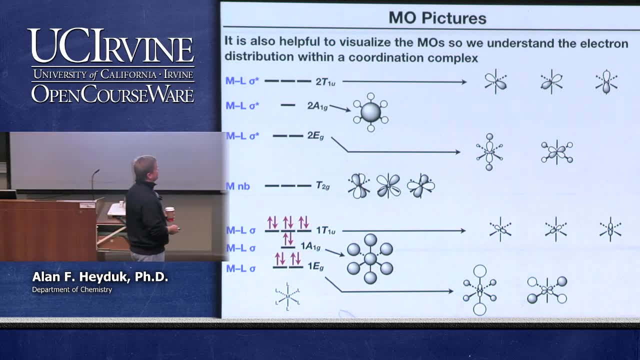 on the metal. Finally, we have the T1U. We know that the metal contribution here are the PX, PY and PZ. The ligand is going to make in-phase contributions with the same nodal properties to the bonding orbital. 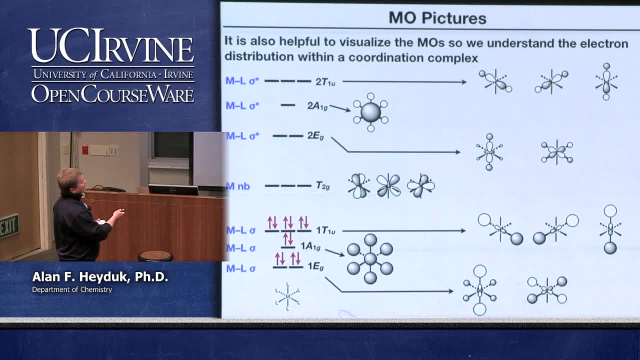 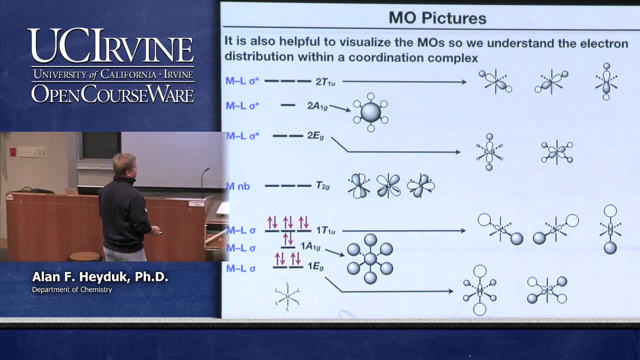 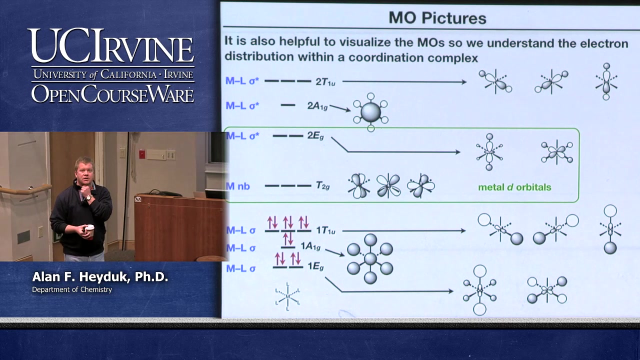 Out of phase contributions to the anti-bonding orbital. Again, the metal ligand bonding orbital is localized on the ligand. The metal ligand anti-bonding orbital is localized on the metal. Now, if we look at these pictures, we see that we have a block of orbitals right in the middle. 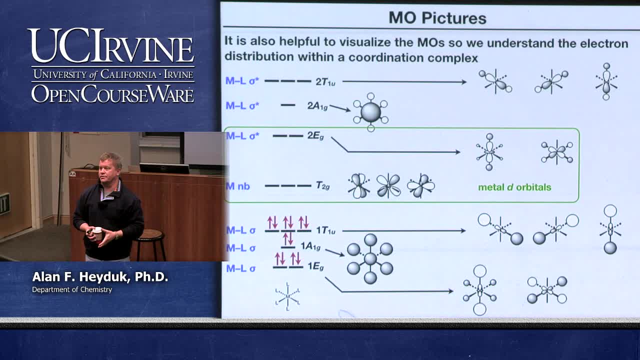 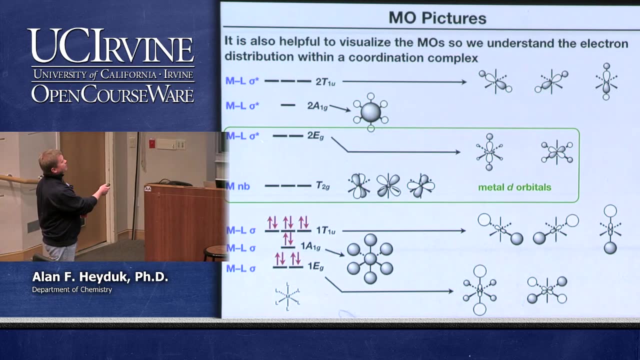 that are dominated by metal D character. The T2G, that's all there is at this point, is metal D character. Those are pure D orbitals. at this point, The 2EG, this metal ligand sigma star, well, we said, 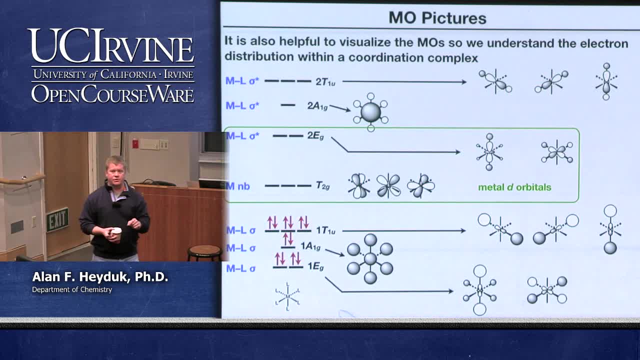 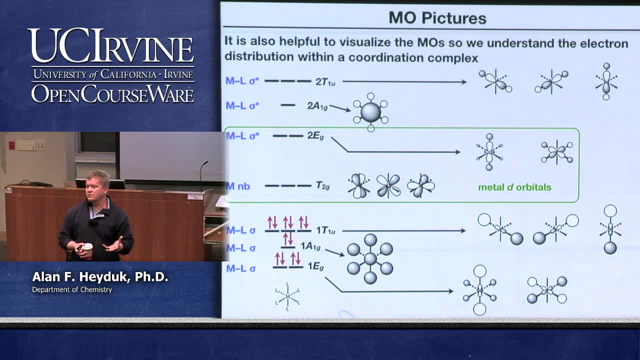 that that's localized on the metal. It has a bigger contribution from the metal than it does from the ligand. We make the approximation, then, that it's essentially a D orbital. It's not a pure D orbital, but it's mostly D orbital. 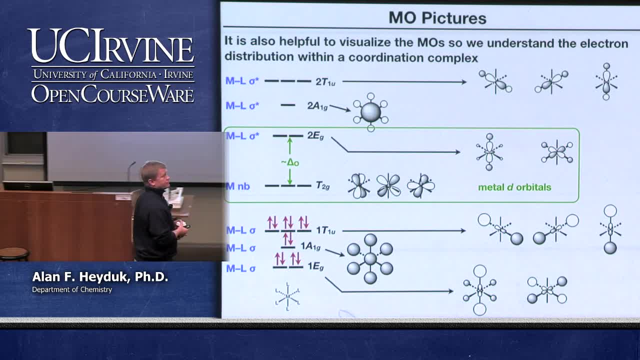 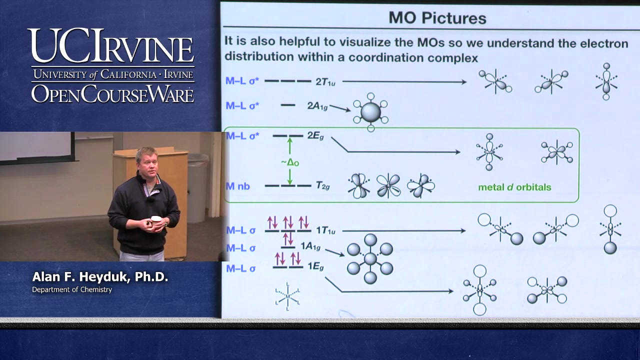 in character. That separation that we just got from molecular orbital theory looks a lot like the separation we got from crystal field theory And to a first approximation it is. We can call that separation between the T2G metal non-bonding orbitals. 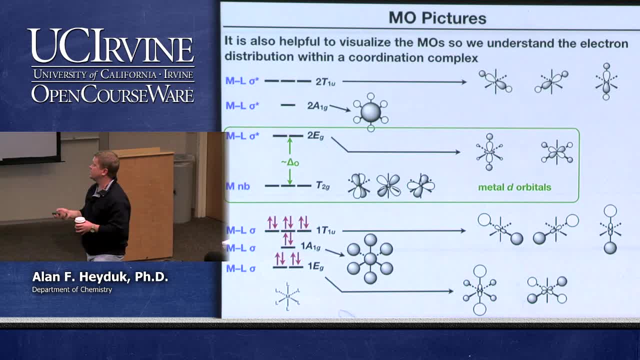 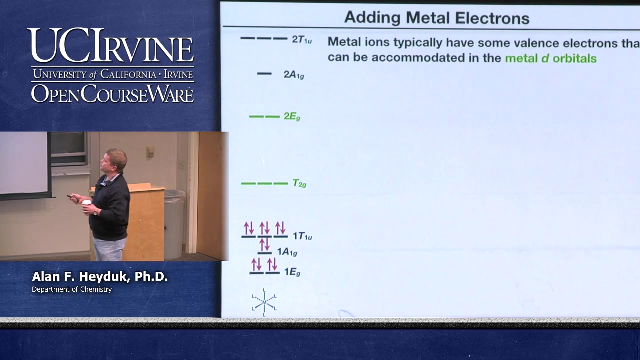 and the EG metal ligand sigma star orbitals. we can approximate that as delta O. Delta O has some other things in there that we'll get to eventually, But to a first approximation that's a legitimate label. Okay, so here's our orbital structure. 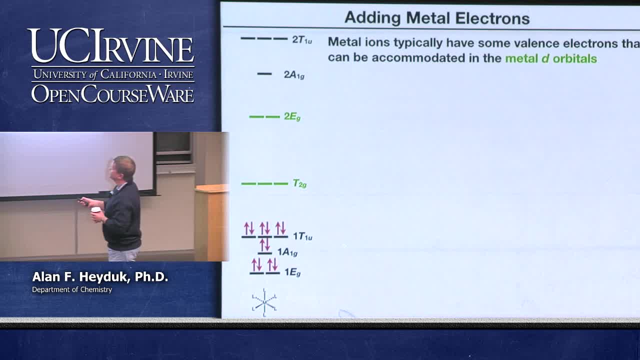 for an octahedral complex. Again, I'll remind you, these are the six metal ligand sigma bonds. these are the six metal ligand sigma star and the ones in green are the metal D orbitals. It's really important that you remember that this 2EG. 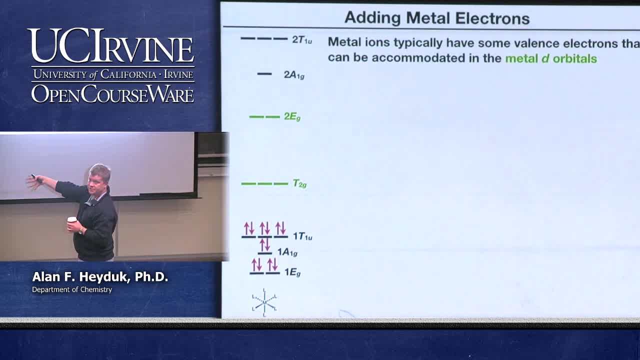 this is the D orbital. Those are both metal ligand, sigma star and considered to be metal D orbitals. Okay, they kind of get this dual label And so we can go in and start to put in electrons according to the D electron count. So D0 metal ions are real easy because there's no D electrons. So it looks just like that You always have to have Okay, So you have to have Okay. So you have to have six pairs of electrons in metal ligand. 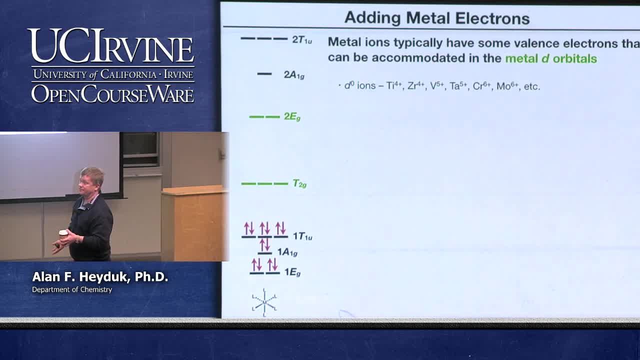 bonding orbitals to have six ligands coordinated to the metal. If you don't have six electron pairs down there, you don't have six metal ligand bonds and you can't have six ligands bonded to the metal D1, one electron goes in T2G. 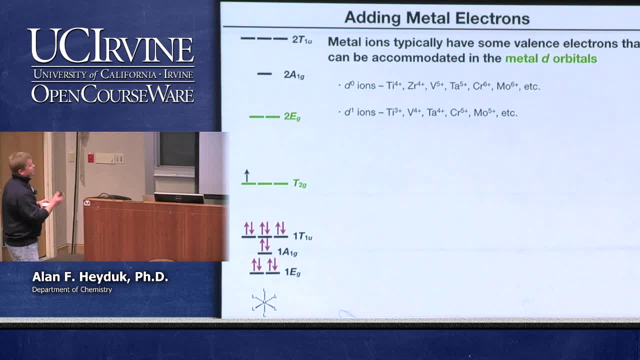 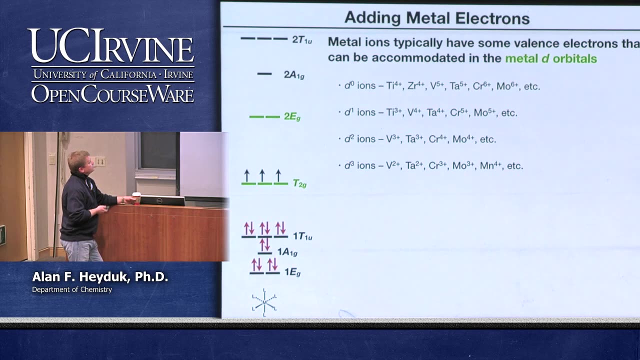 Common examples: titanium 3, vanadium 4, so on and so forth. Okay, The D2s. we're just following the Pauli exclusion principle and Hund's rule. Two electrons spin up into the T2G D3, you have three unpaired electrons all spin. 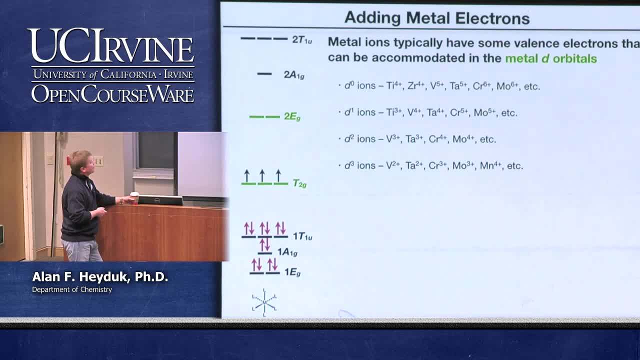 up all in the T2G orbitals. Now we're going to pause. We're going to skip over D4, 5, 6 and 7 electron counts. We're going to come back to that. We're going to come back to those on the next slide. 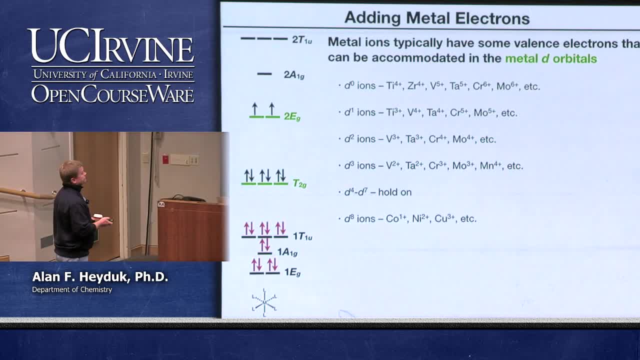 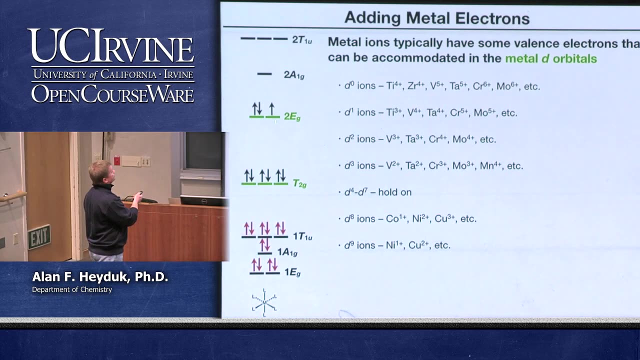 If we get to D8, the only way to put the eight electrons in is to fill T2G with six electrons and have two electrons in EG D9, examples are nickel 1, copper 2.. We end up with a total of three electrons in the EG. 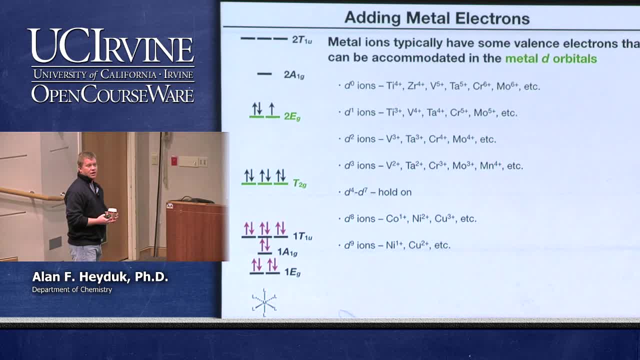 Remember, this is a metal ligand anti-bonding orbital. It's kind of interesting, right, Because if we start populating anti-bonding orbitals in an organic, complex well, things start flying off right. You abolish the bond. 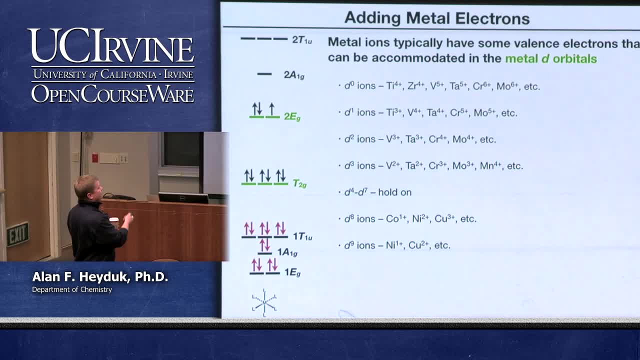 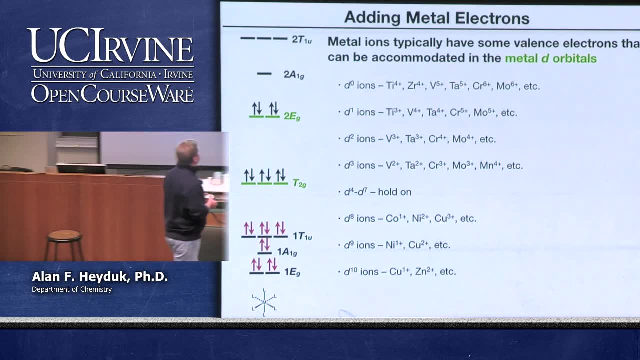 Transition metal complexes. we can populate anti-bonding orbitals and the ligand still stays on. There are even octahedral D10.. You take zinc 2 and you dissolve it in water. six water ligands will coordinate. They will coordinate to the zinc. 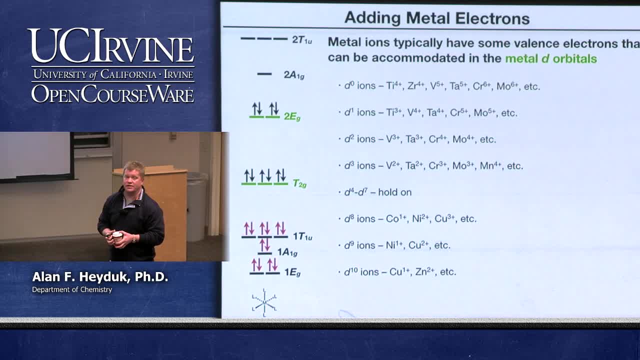 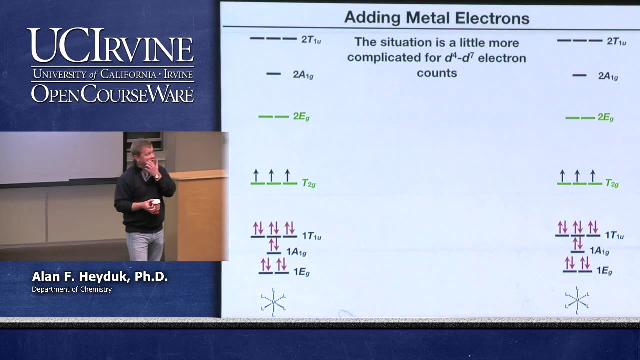 But it's kind of again kind of interesting because technically the anti-bonding- we have four electrons in anti-bonding orbitals And it does that does have consequences for reactivity. Okay, what about those other D4, D5, D6, D7?? 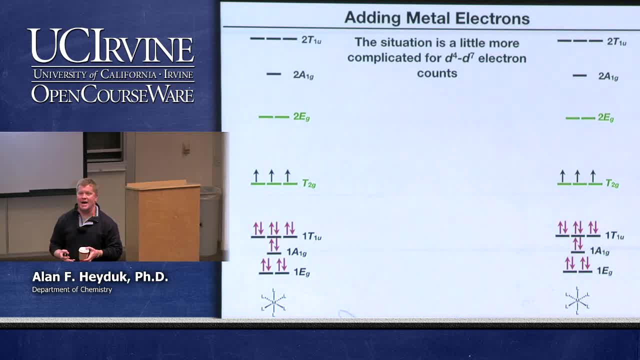 It turns out. this is where we come back to that idea of high spin versus low spin. Okay, There's two different ways that we can put four electrons in the D manifold, And so examples of D4, chromium 2, molybdenum 2,. 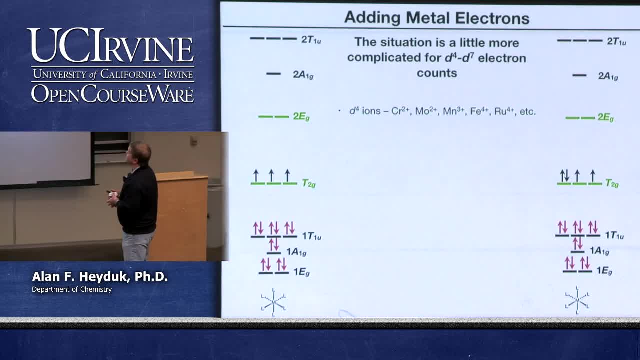 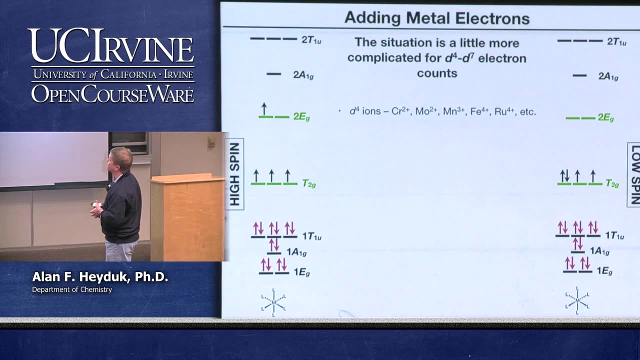 iron 4, so on and so forth. You can take and put one electron and pair it down here in T2G, or you can put one electron in the EG orbital. That gives us again our designation: high spin electron configuration or low spin configuration. 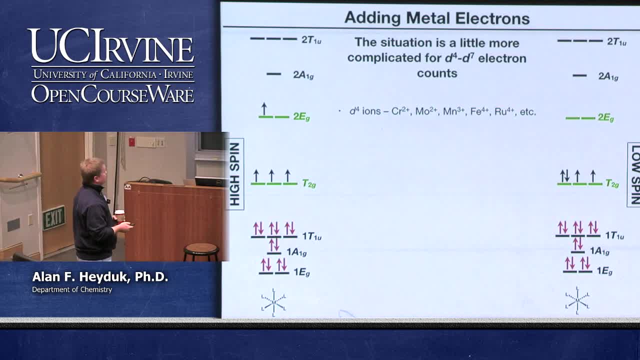 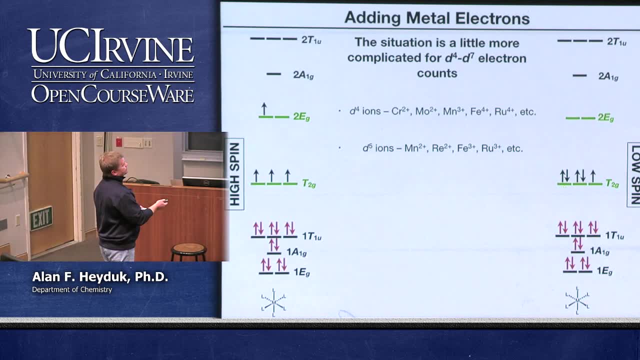 I promise I'm going to teach you how to predict which. it's going to be D5, same thing. If we continue putting electrons into T2G, we're going to get a high spin electron configuration. If we continue putting electrons into T2G. 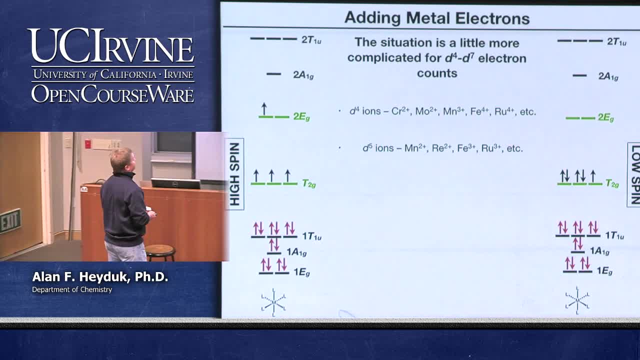 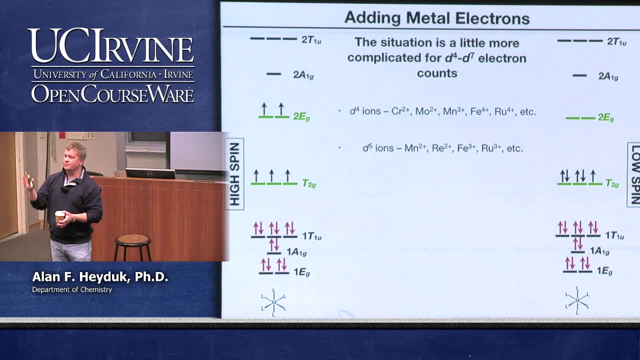 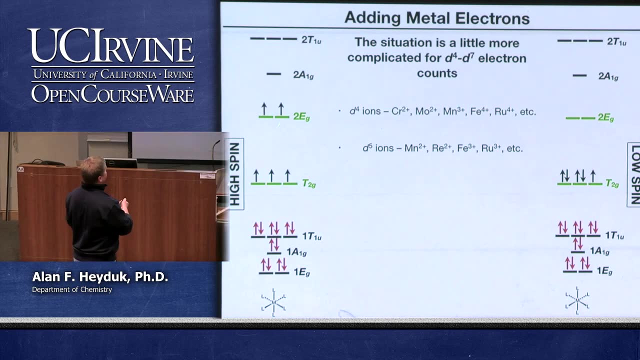 we pair what we make another pair for the low spin, For the high spin we put an electron up in EG. Now we've reached our maximum number of unpaired spins in a octahedral complex right, Because there's no more places to put spin. 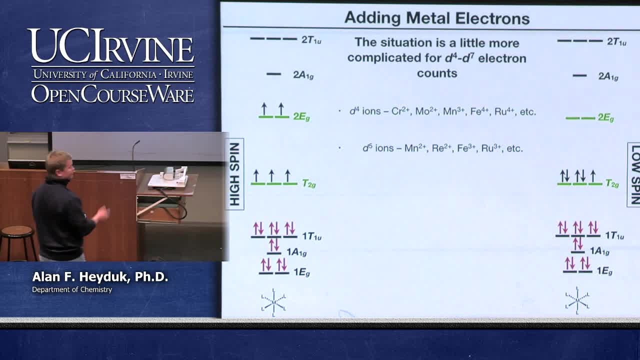 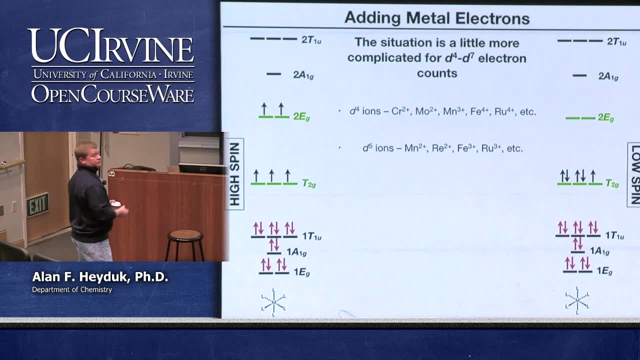 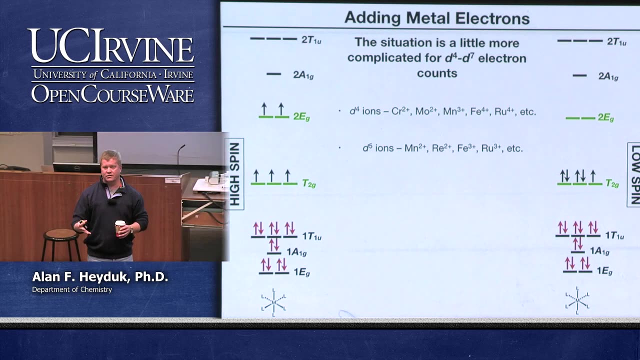 up electrons in the D orbitals. You will never, ever, never, period, like never, never, ever, put an unpaired electron up there. It will not happen ever. You know those rules that are made to be broken. This is not one of them. 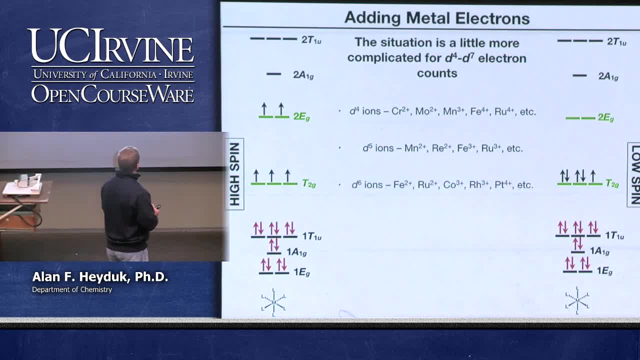 It never happens. okay. D6, the low spin case is kind of satisfying because you basically form a closed shell. D6 octahedral complex. What would be an example? O, platinum IV- Remember I told you if I see platinum in an octahedral field.